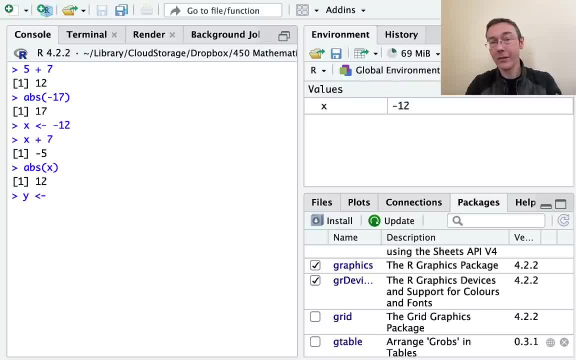 You can also assign x to be the absolute value of x. I'm sorry, Variables to be entire vectors of values. Let's let y be equal to negative 12,, 6,, 0, and negative 1.. You can see now I have a value stored for y, but there's actually four numbers in there. 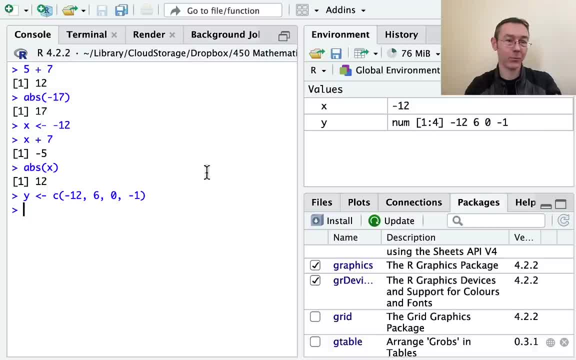 It's sort of an ordered n-tuple: Negative 12,, 6,, 0, negative 1.. I can do operations on y, on this vector, For instance, I can double the whole thing. Notice that's happening. component wise, i can apply functions to it like absolute value of y and expect those. 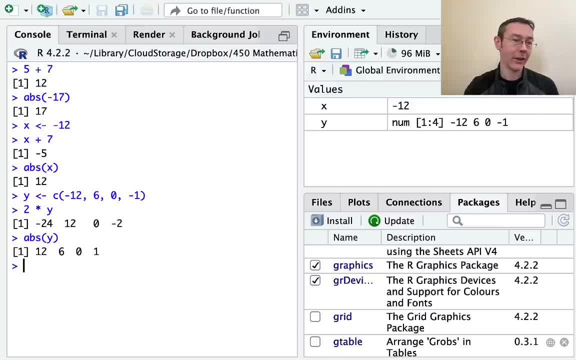 to be done. component wise, i could take a sine, a tangent, an exponential, whatever i like. if you're watching this video, though, you're probably not so much interested in the programming aspects and more on the data aspects, and that makes sense. r is fundamentally a language set up for working. 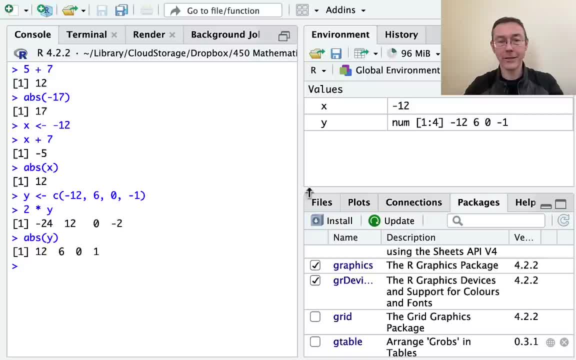 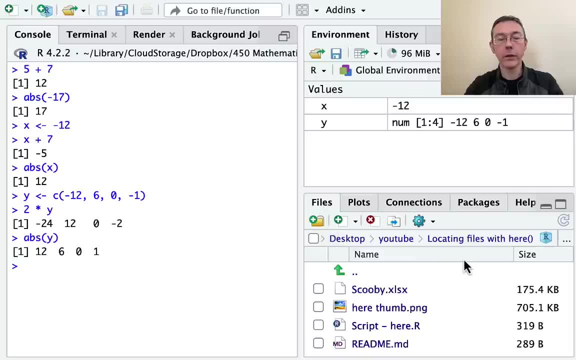 with data. so let's import a data set and and take a look at it. here in the lower right i have a file browser, so i'll click on that and you can see. you can navigate around your machine until you find the data set that you want to work with and, if you have an excel spreadsheet, for instance, or a csv, 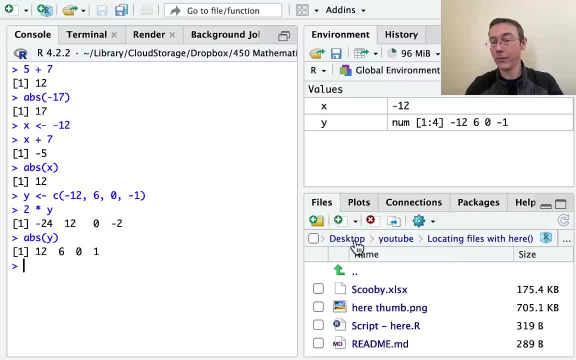 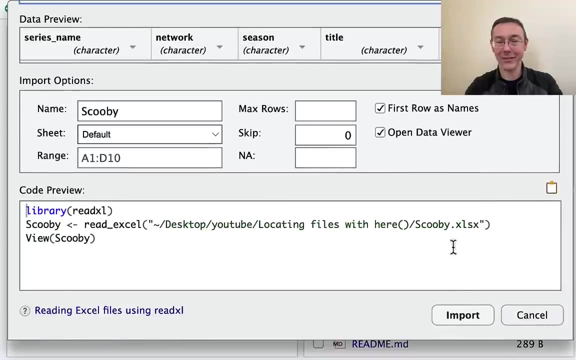 file. importing a data set is extremely easy. just find it by following these breadcrumbs, clicking on the folders that you want, and then just click on the file that you want and go to import data set. that'll pull up a window with lots of different options that you can more or less just ignore when you're getting started and just click import. 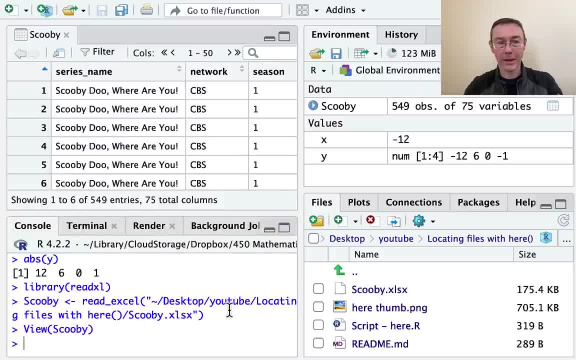 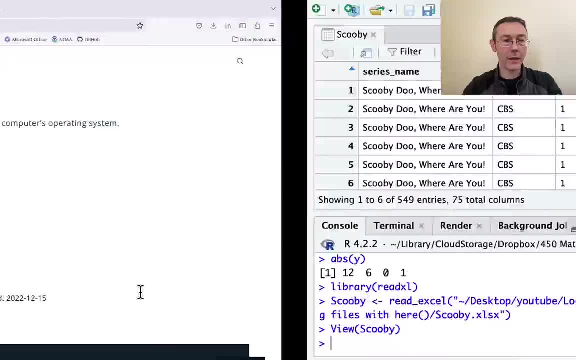 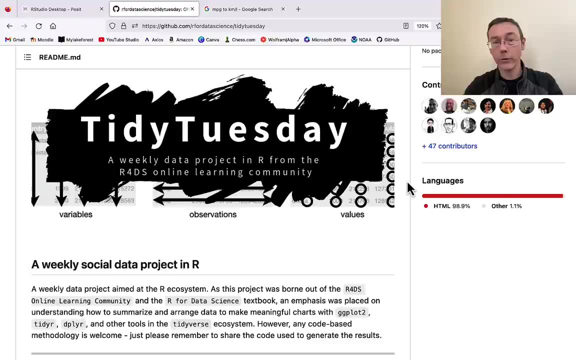 okay, so a few things have happened. before i talk about any of them, i just want to mention that what this data set is that we're looking at this is the scooby-doo database, and i got it from the tidy tuesday project. every week, tidy tuesday posts. 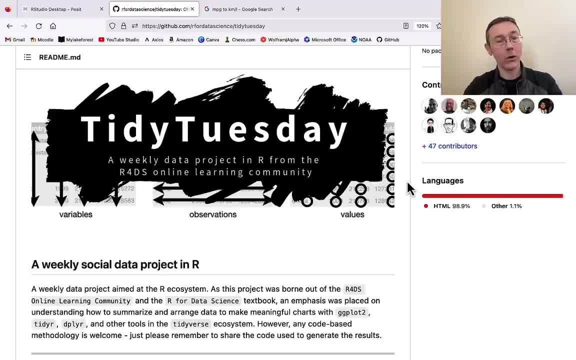 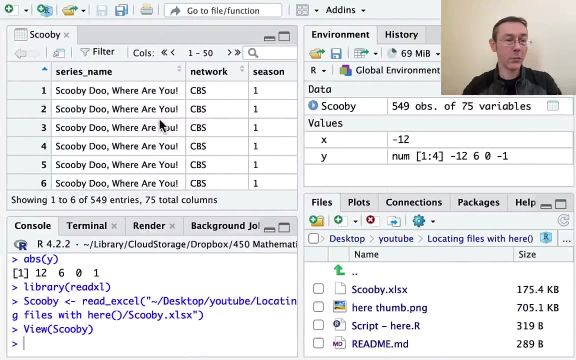 a new and interesting data set for us to practice our our skills- data cleaning, visualization and analysis more broadly. you can also, of course, work with these data sets in other languages, but this definitely is revolving around the r ecosystem. strongly recommending this to check out. tidy tuesday: the scooby-doo data set was featured at one point or another. okay, back to the. 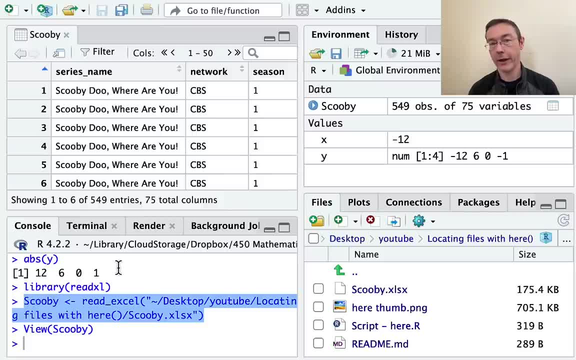 next slide. so the import is actually happening here. in the second line, the read excel command and you can see inside it has found the file in question. you can see the file path there, read it in and assigned it to the variable named scooby. and if you look in my environment, tab up here: 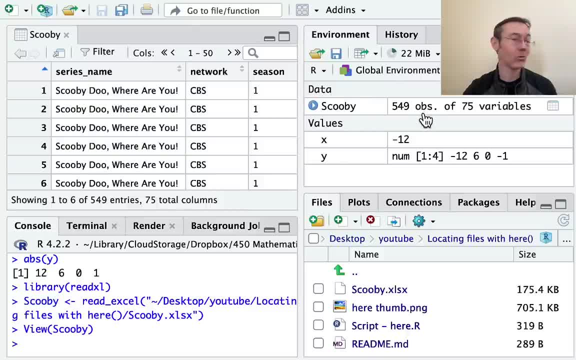 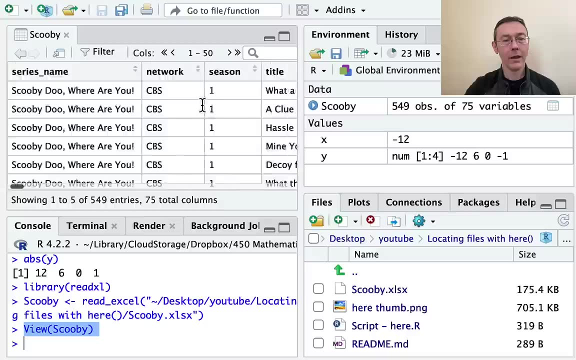 on the upper right there's now a data set- 549 observations, rows of 75 variables, columns- and you can see that the view command is what actually opened up that data set so that we could see it. it actually just put it in the viewer in an interactive way and we can kind of scan. 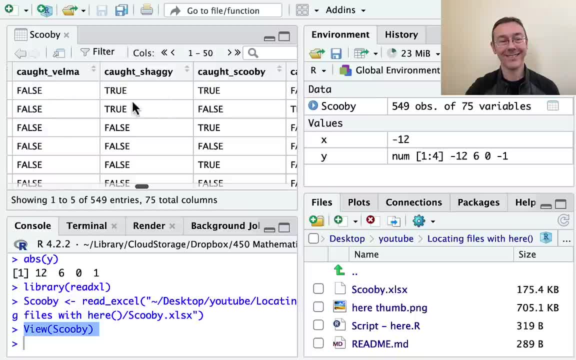 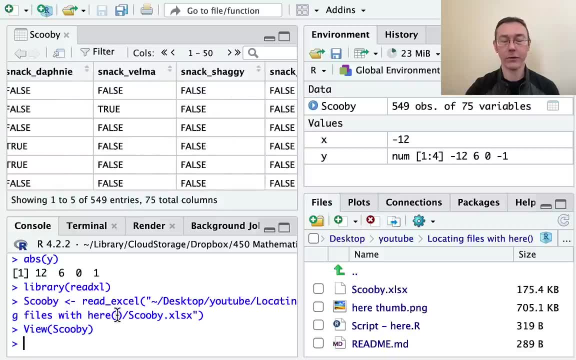 through it and see some of the variable names. who caught the villain, velma shaggy and so on. did shaggy get a scooby snack? stuff like that, lots of fun stuff here. this first command library- let's talk about that for a second. the library command is an old language but over time it has been expanded and developed by its 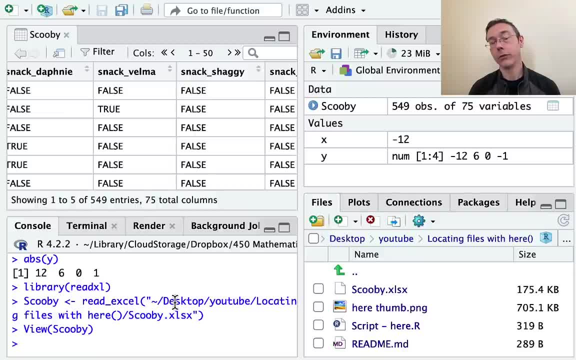 large and vibrant community of users. the add-on sets of functions that they have created and which are available to us are called packages, and this library command is opening up a package of functions called read excel that give us some additional functionality for working with excel spreadsheets. you can think of this package, read excel, like an app on your mobile phone and the 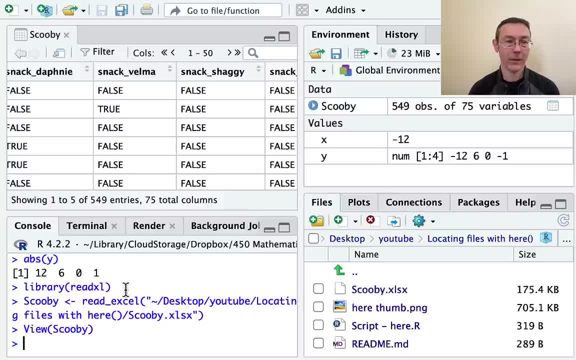 library command app and giving us access to its functions. but if you haven't already installed that app, if you haven't already installed this package of functions, r is not going to know what to do with this library command, won't know how to open the app, so you need to start by installing it with install. 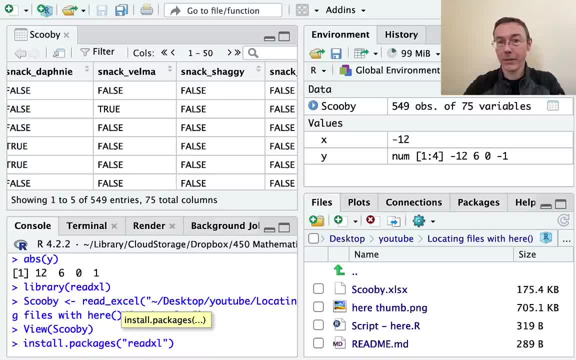 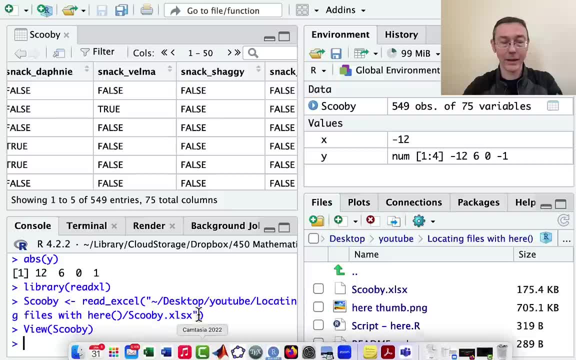 packages- parenthesis- quote: read excel. i won't actually execute that because i already have it installed and actually i already have the package loaded, so that's not something i need to do. you only need to install the package. you don't have to open it once, but every time you want to use it, every session, every time you open. 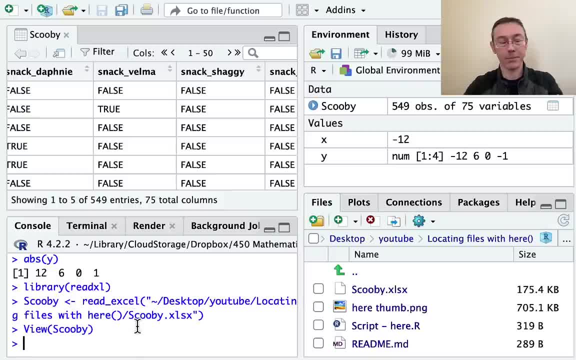 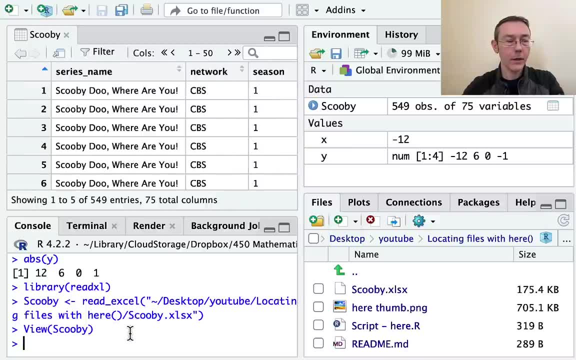 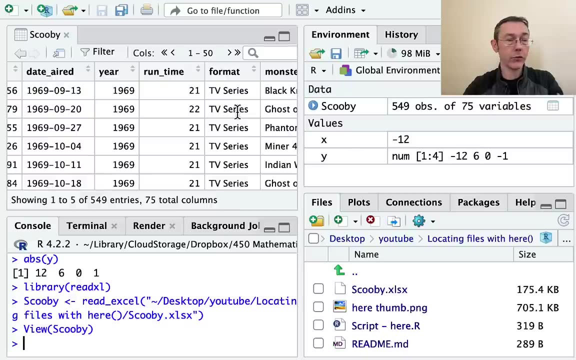 up r and want to use it, you have to library it, you have to actually open that app. okay, so lots of interesting stuff here, lots of interesting variables. um, we might want, for instance, to get some summary information on some of these variables, like, for instance, what's the average run time of all the episodes in this database? 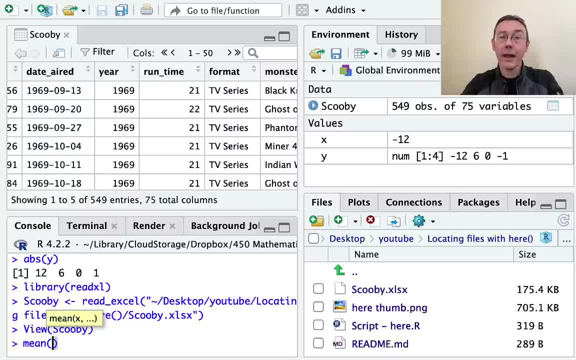 not surprisingly, that's a mean command. Now I want to get the average of this column in the scooby data set and the syntax in R is to first name the data set. so scooby notice the autocomplete suggestion. you can either use tab or enter to acknowledge that. So I want the mean in the scooby-doo data set of the. 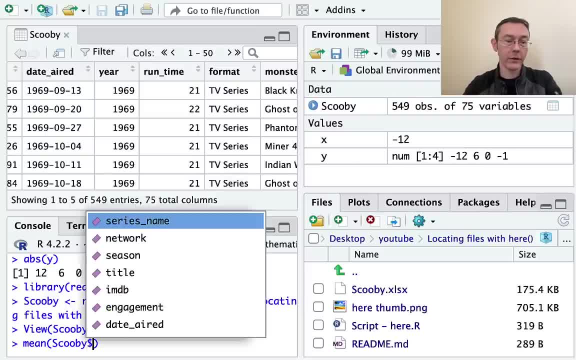 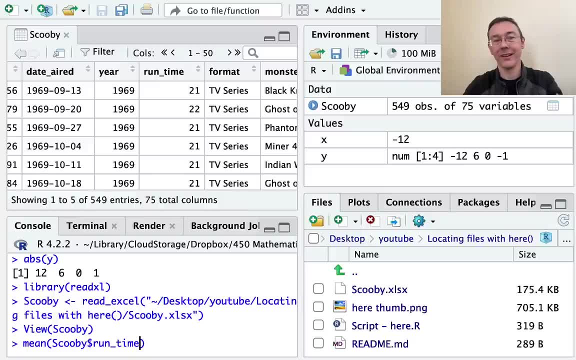 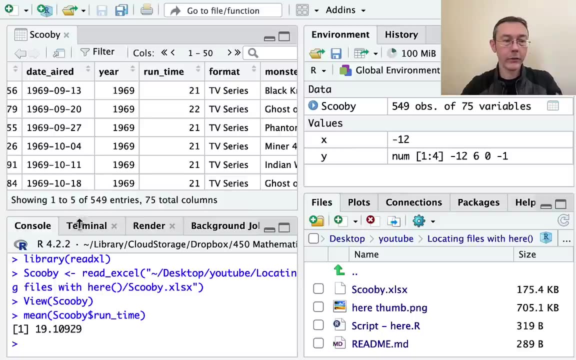 runtime variable and I'll specify the column I want with a dollar sign, and then, if I start typing runtime, I can then select the variable that I want or just type it entirely. A little more than 19 minutes for the average runtime of all these episodes. Let's do the same thing for IMDB: the average IMDB rating. 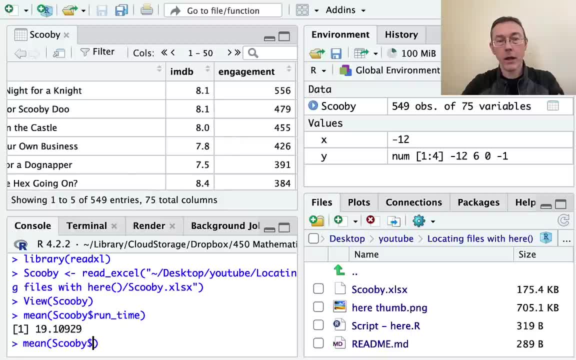 we'll see. there's a little bit of a subtlety. Notice how fast I was able to key that in. I used the up arrow to get to the previous command, and if I want to get two commands back to the previous command, I can do that by clicking the. 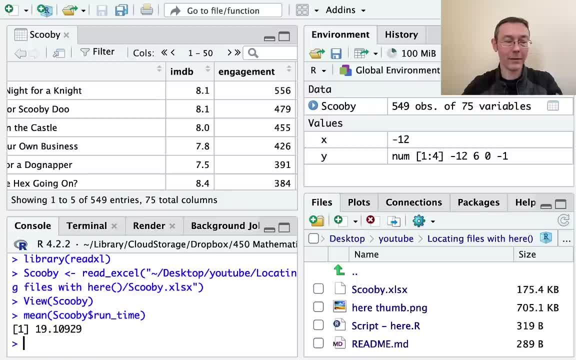 back. I go up arrow twice so this can save you some time, some typing time. so up arrow and then back, spacing over runtime and I'll replace it with IMDB and when I execute that to get the average IMDB rating of all these episodes I get. 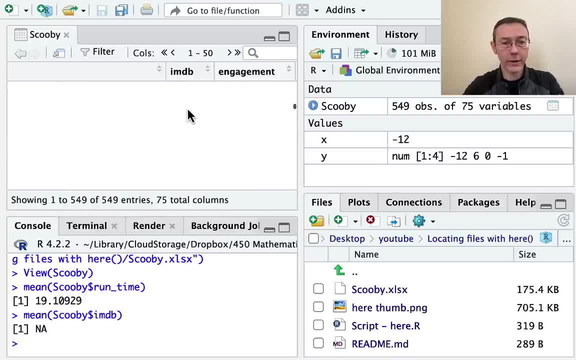 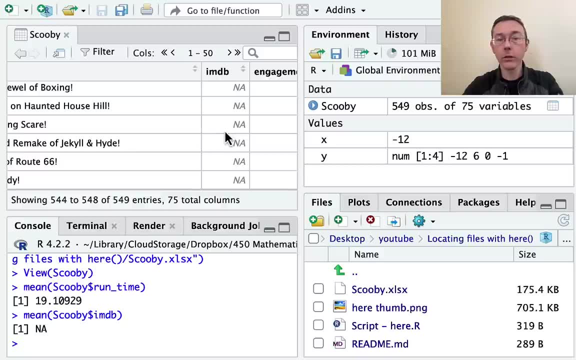 an N? A, and the reason is, if I go all the way down to the bottom here, there are some N? A's in this column, Some missing values. there's literally nothing missing. So I'm going to go back to the previous column and I'm going to 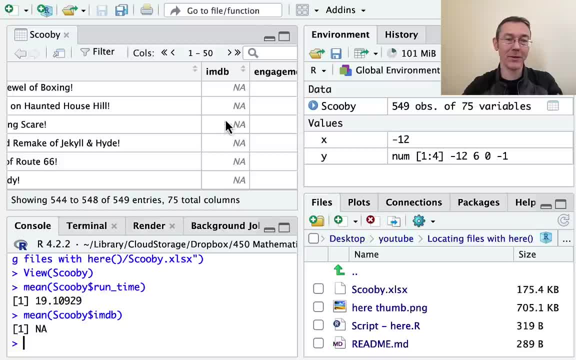 search for those. and that's just a piece of data and we're going to do some fast forward projection. at the bottom of the column, As you can see, there's no data for more recent episodes of Scooby-Doo in here. They just didn't have. 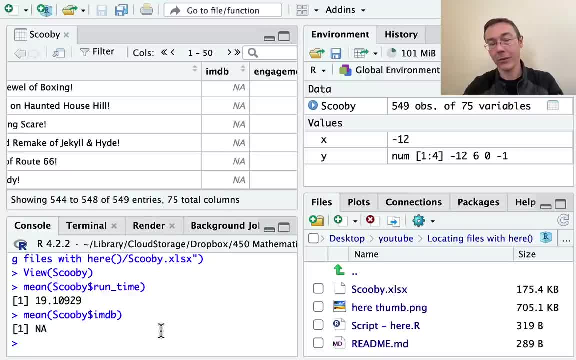 IMDB ratings when this set was made, and so when R tries to figure out what the average IMDB rating is over time, it just doesn't know, because these n A's could be very high or very low, and so those N A's propagate. So the mean command I'm 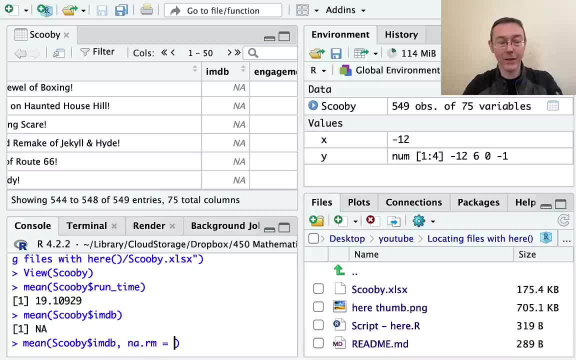 using the up arrow here. like many functions in R has optional arguments. remove the NAs is true. You can leave out narm and it will default to false. Leave them in. Here I'm overriding that and saying take them out. The average IMDb rating in this set. 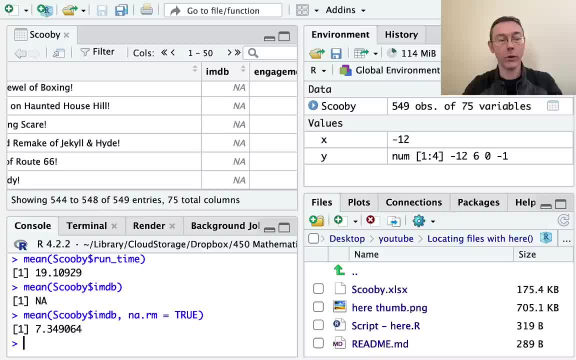 for the episodes that actually have IMDb ratings is 7.34.. Okay, now we've already done a bunch of commands here. Things are starting to get a little bit busy. If you're doing a more full data analysis going line by line like this can be problematic. 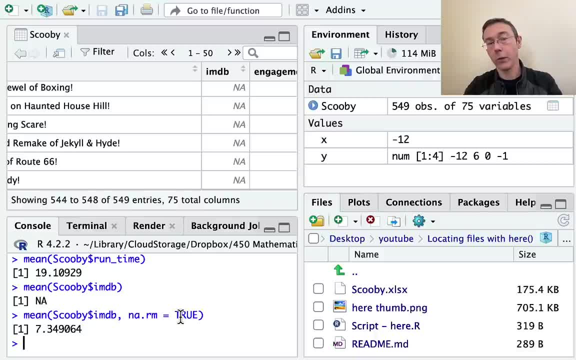 You can lose track of your work. It's also more difficult to recreate things later on, So what we'd like to do is to actually have a document that actually encodes all of this, that actually contains all of this. In this video, we're gonna see two ways. 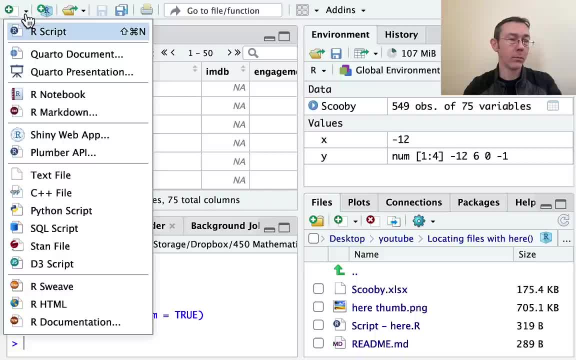 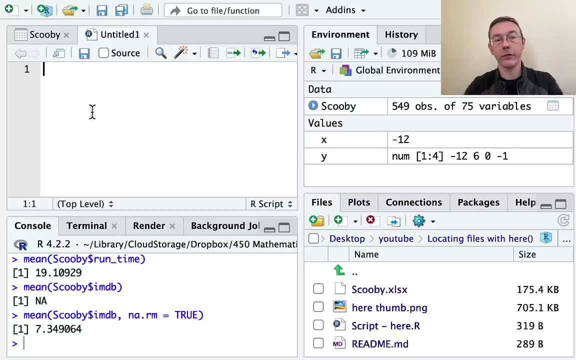 The most fundamental, though, is a script, And so I'm gonna go up to this little piece of paper here and get new R script, And that's gonna open up a new tab right next to my data set. That's essentially just a text file. 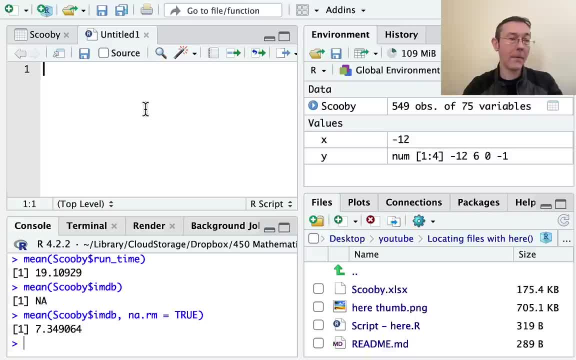 And the idea is that we can code line by line here and then save this file later on just using the disc icon, and save it anywhere we want. So, for instance, I could put in a library command like library read Excel. Going forward, I'm going to wanna use an entire ecosystem. 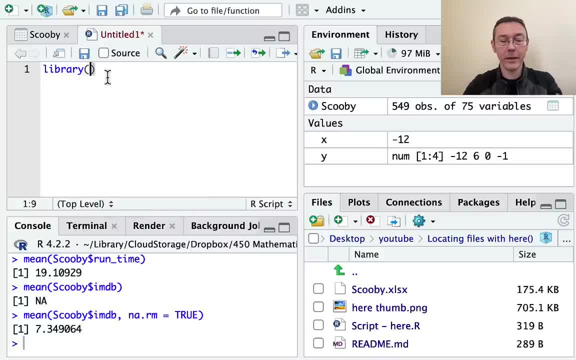 of packages that have become, excuse me, very popular over time, And that is the Tidyverse family of packages. These are produced by Posit, the same company that makes this front end RStudio, largely developed by their chief data scientist. 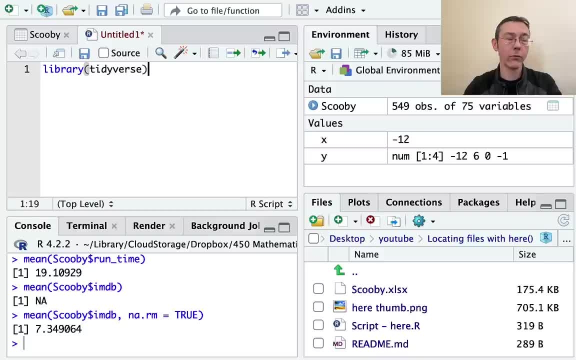 Hadley, Wickham And the Tidyverse family of packages have really revolutionized R and data analysis just over the last decade, So I'm gonna execute that. If I just hit enter right now, nothing's actually gonna happen, except I'm gonna get a new line. 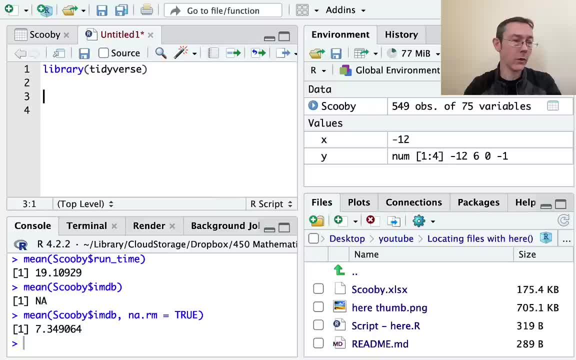 This is literally a text file, And so R doesn't know that I'm actually wanting to execute that code. It just thinks I'm wanting to go to a new line to write some more stuff. If I wanna actually execute the code, I have to hit command enter on a Mac, which I'm on, 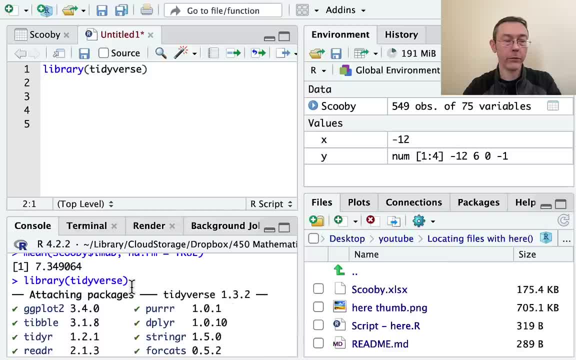 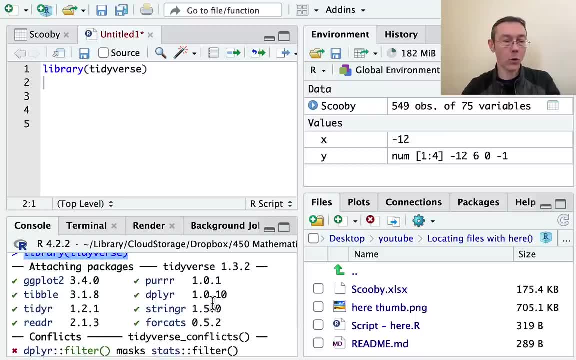 or control enter if I'm on a PC, And then that will send the line of code down to the console and actually execute it. The Tidyverse consists of eight core packages. You can see them listed here. They all have some pretty important purposes. 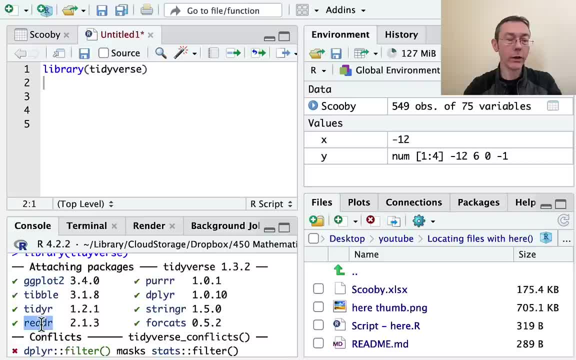 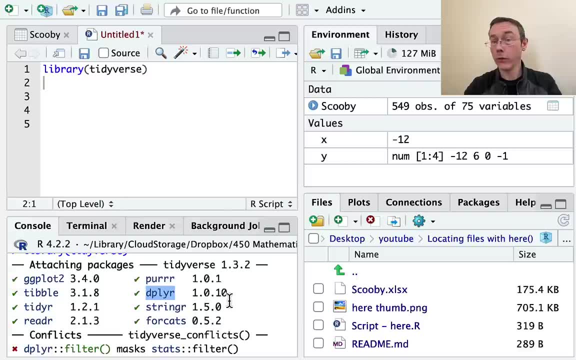 in R. I would say that ggplot2 and dplyr in particular have become absolute standards in R programming. If you are using R today, you absolutely have to know those two. The others have been largely adopted as well. It's certainly worth learning them all. 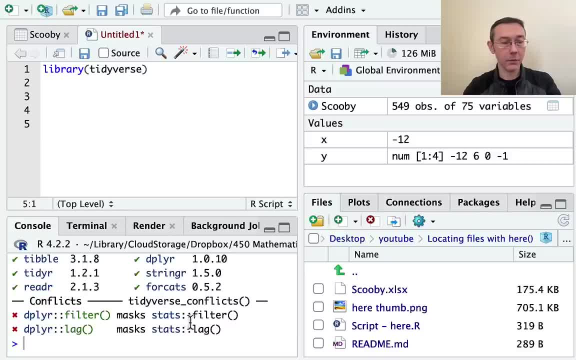 In this lecture, in this video, I'm gonna talk about those two packages a little bit. I don't think I'll get into any of the others particularly Okay. The first command I wanna show you other than loading up packages, or the first, I think, helpful tip I wanna point out: 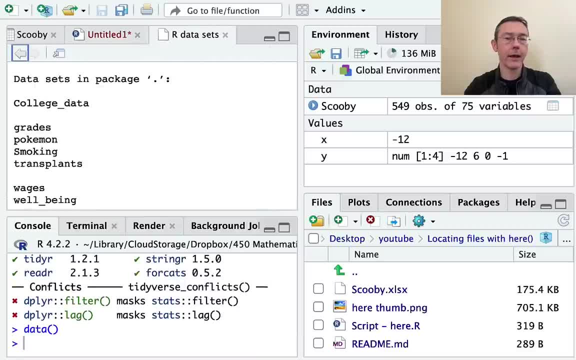 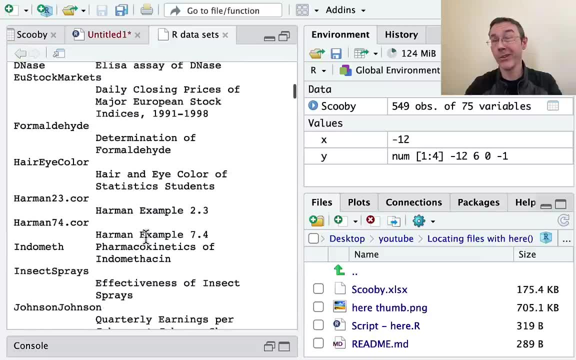 is this data command And I'm gonna hit that And when it happens, when I do that, it's gonna show me a long list of data sets that are built in in R that you can use to practice some of the skills that I'm gonna be teaching. 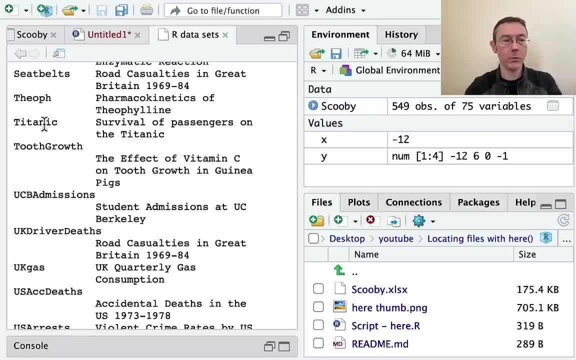 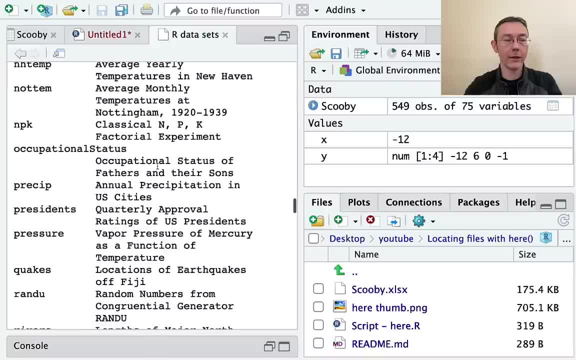 Some of them that are just built in with base R, that just come, no matter what else you do like- Titanic is a famous one- And some that load up with these other packages. So, for instance, if I scan down far enough data sets in the package dplyr. 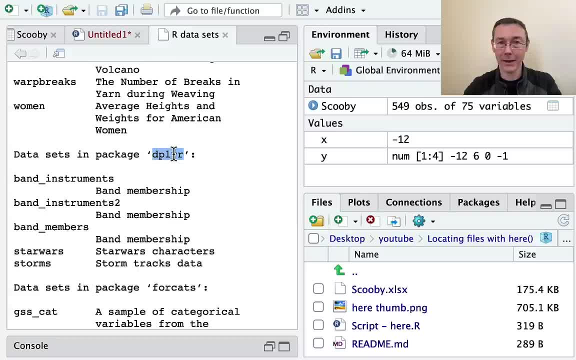 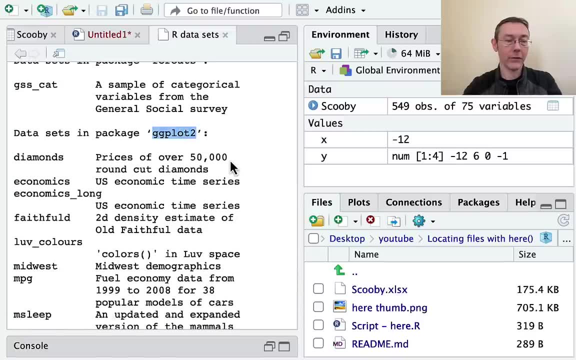 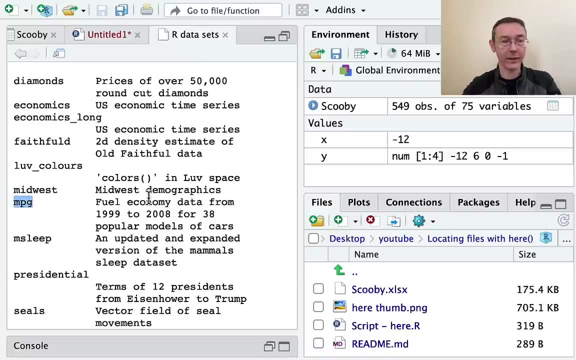 So these are some data sets that are included with that dplyr package that was included in the tidyverse that you can use to work on your data wrangling, ggplot2 and so on. In the next few examples I'm gonna be using the mpg dataset. 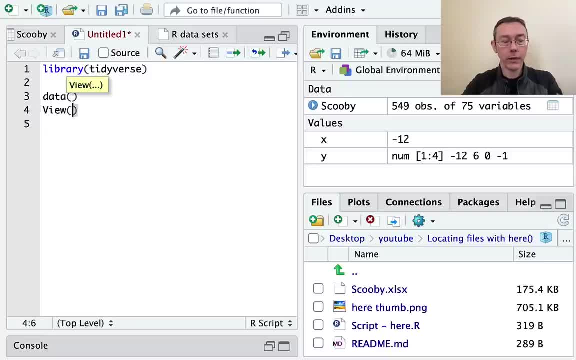 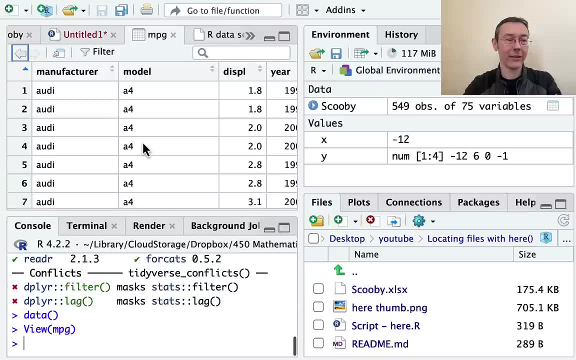 So I could do view mpg. We've already seen that command when we imported the scooby dataset. I'll hit command enter to actually execute it And you can see. the command was sent down here And now the mpg dataset gets opened up in the viewer. 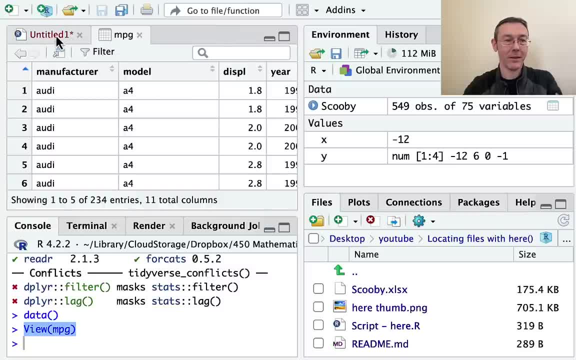 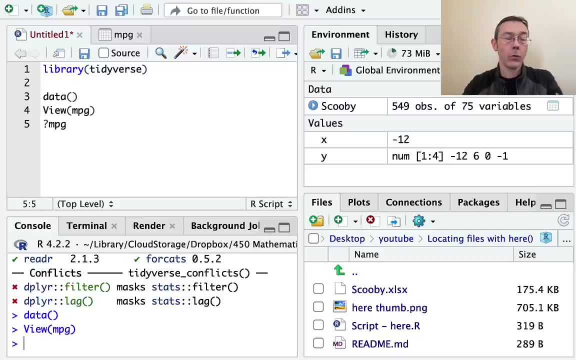 I'm gonna close up a couple of these other windows for neatness. Okay, so I don't know anything about the mpg dataset. I wanna learn a little bit more about it. When you want to learn more about a function or a dataset that is either built in or loaded in with a function, 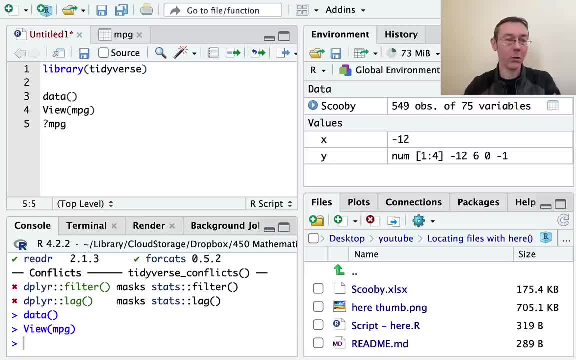 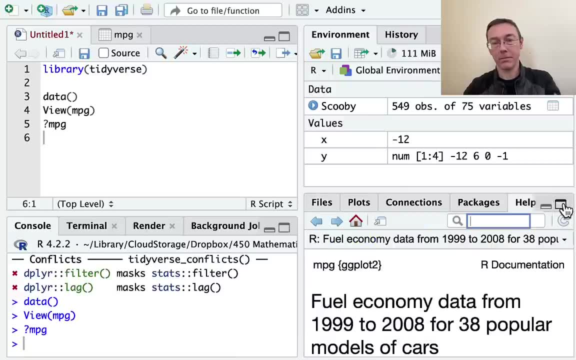 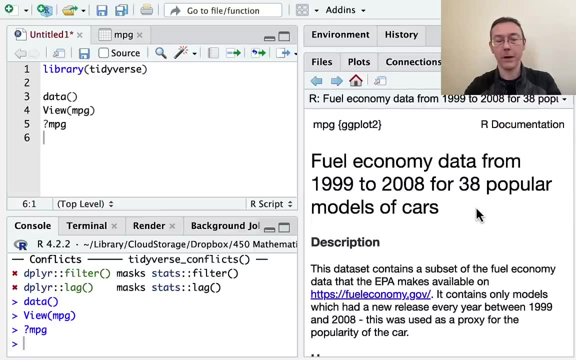 or loaded in with a package. you can ask about it with question mark, in this case mpg, And when I hit command enter, that will open up something in this help tab. In this case we see we have fuel economy data from 1999 to 2008 for 38 popular models of cars. 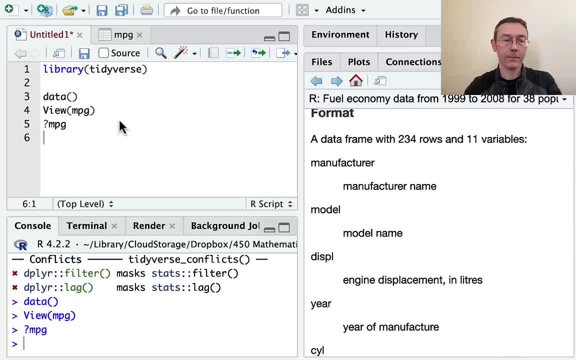 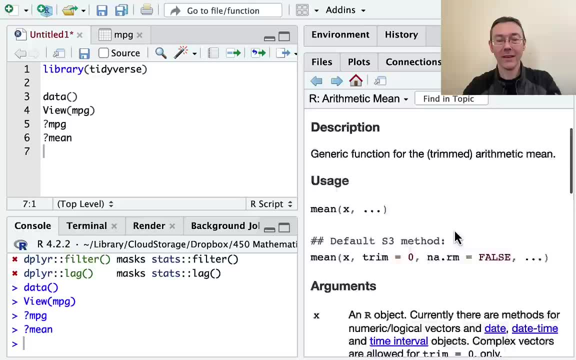 And then we have a little bit of a data dictionary telling us more about it. We can get help files on all sorts of functions, as I mentioned, for instance mean to get the arithmetic mean And you can see the sorts of arguments we might use. 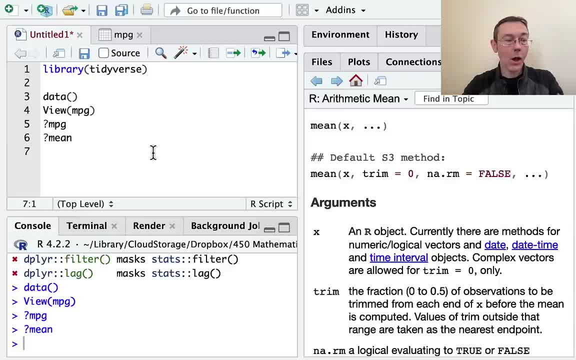 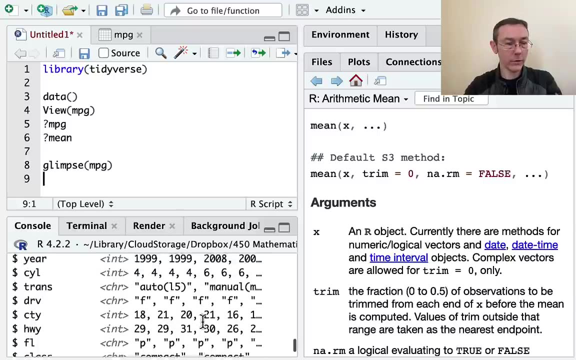 as well as some of the optional arguments. Okay, one other command I would like to show that I think is very helpful when you're encountering a new dataset is the glimpse command And you just feed it the name of the dataset And the glimpse command. if you look down here, 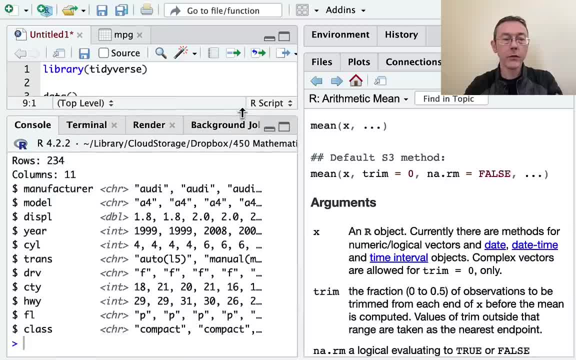 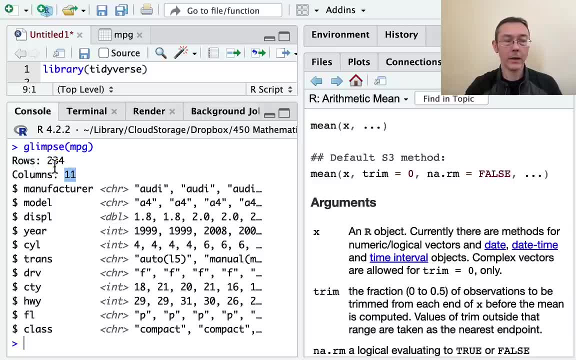 maybe let me make this a little bit more clear. It's a little bit more visible for the moment Just gives you sort of a top level overview of your dataset: How many rows, how many columns, what are the variable names? Remember, after a dollar sign. 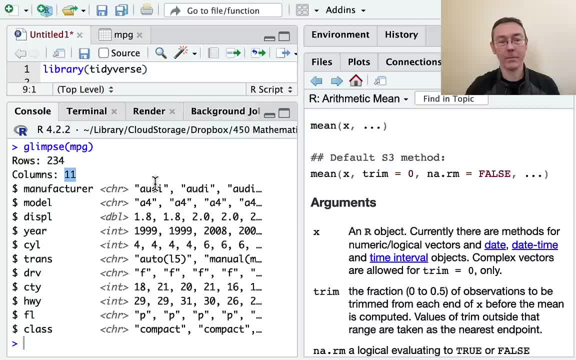 R is typically specifying a variable name in a dataset. What are the first few values And what sort of variable is it? Now, if you have programming experience, you know that different variables can have different types, and you've probably had to suffer. 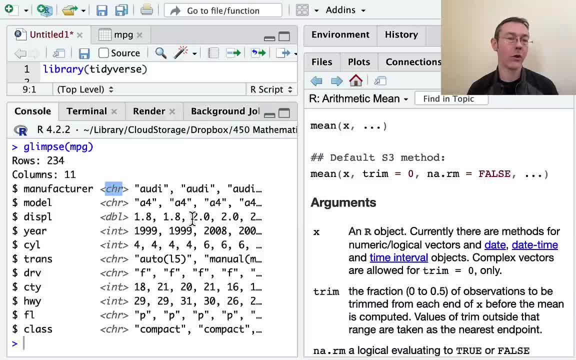 through a fair amount of information on different data types. In R that certainly exists. However, we are able to suppress some of that, some of the technical stuff in our data analysis, and just acknowledge that data can either be categorical, like Audi or A4, or quantitative, like 1.8 or 1999.. 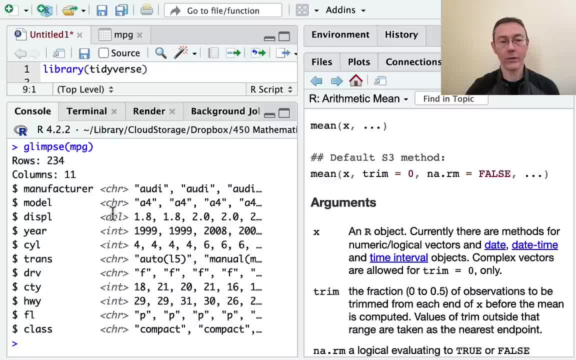 Now at a deeper level of sophistication, there are decimals, doubles and integers. There are factor variables versus character vectors. But another nice thing about R is that fundamentally, for most purposes you don't have to think too hard about that. 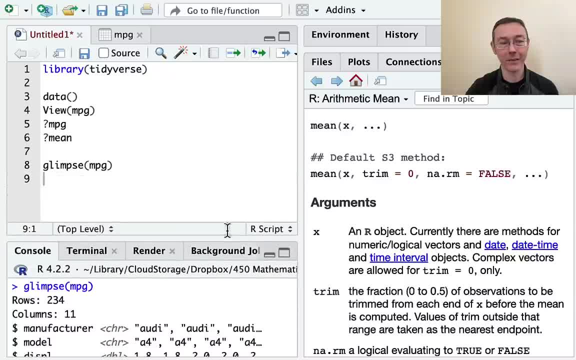 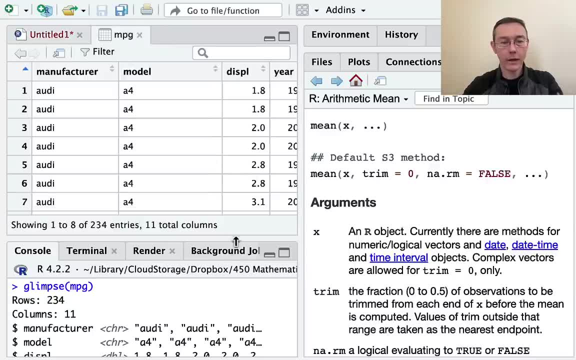 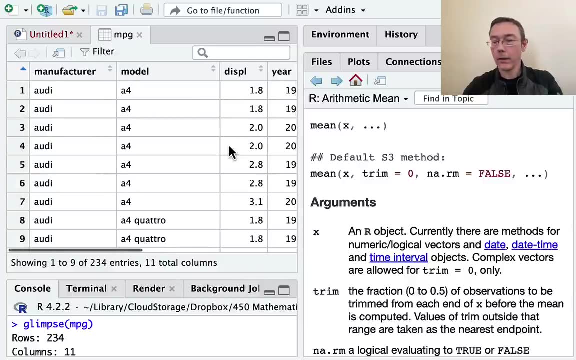 And so I'm not gonna talk anything more about it, not gonna say anything more about it in this video. Okay, so a very common data analysis task that you might have on a set like this is to subset it by rows, For instance. I might be interested. 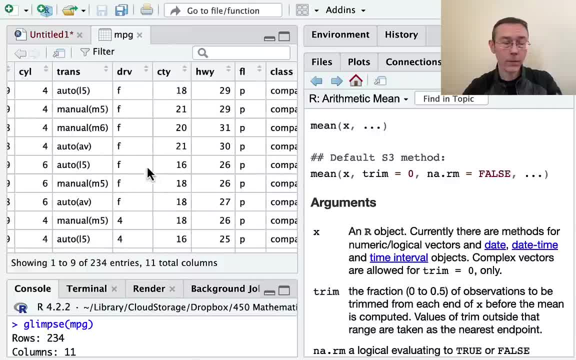 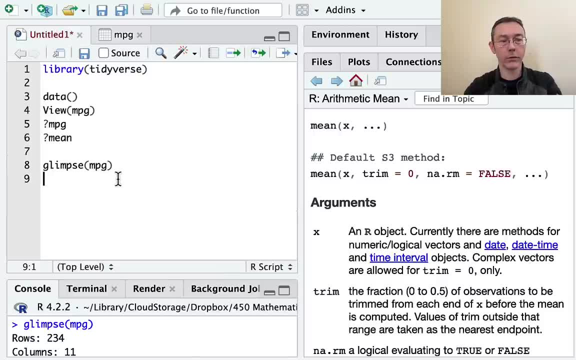 in only the front-wheel drive cars or only the cars that have city mileage at least 20 miles per gallon. So let's do both of those things. The fundamental command we're gonna use to subset by row is the filter command, And of course we can learn more about that. 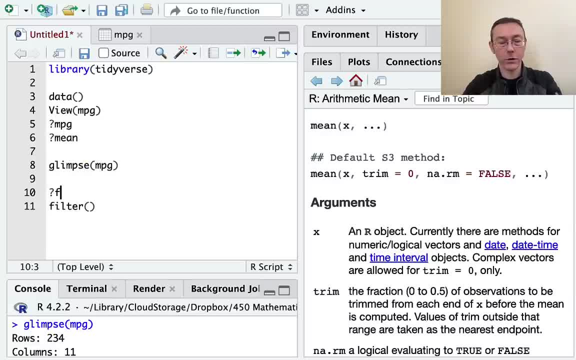 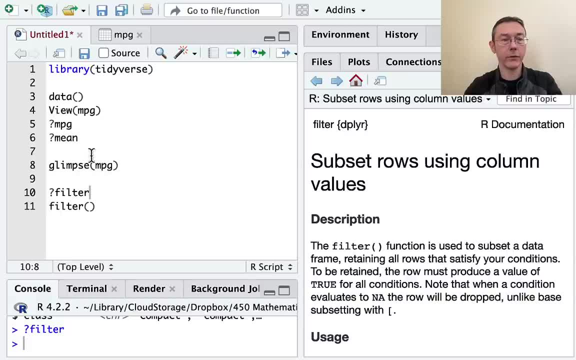 with question mark filter. In fact, maybe I'll just do that question mark filter. So I want this one Subset rows using column values. So, for instance, I'm gonna start out by getting the cars whose city mileage is at least 20 miles per gallon. 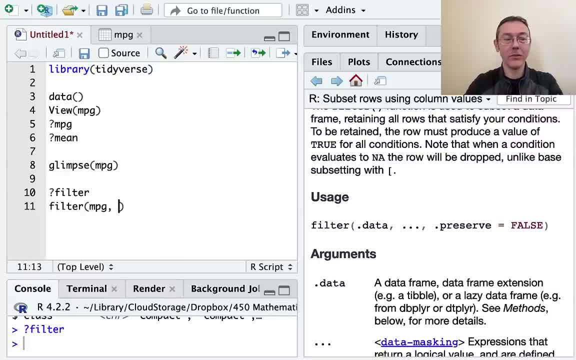 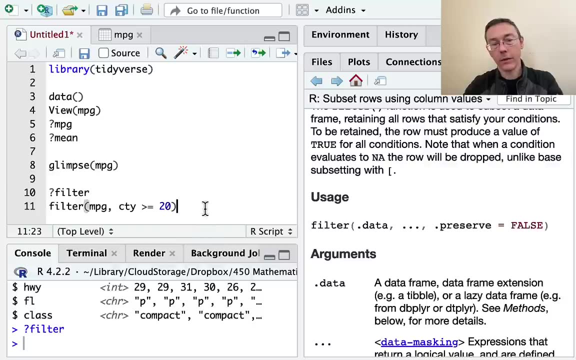 The first argument here should be the data set. So that's mpg. And then I have to specify the condition I want. So city mileage should be at least 20.. So greater than or equal to, And when I command enter this, it's not gonna be exactly what I would hope for. 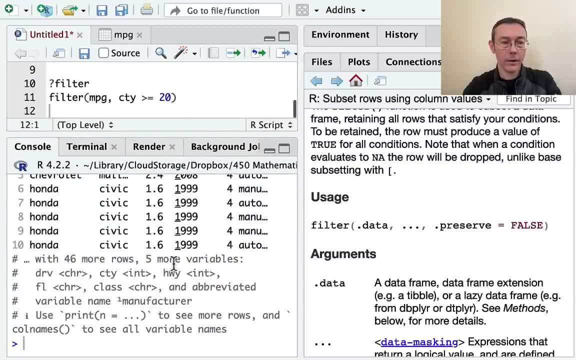 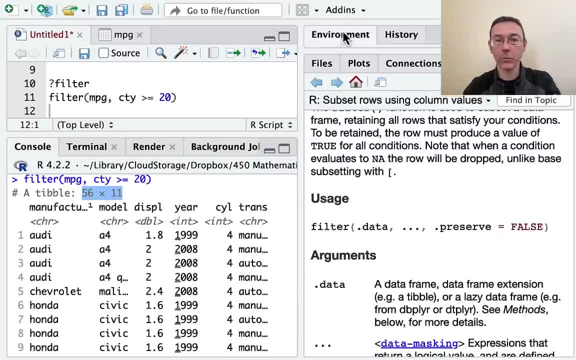 And I'll explain why. Let me get a little better view on this, Okay. So what happened, is it just kind of printed it out. You'll see I now have 56 rows as opposed to the how many did I have before? 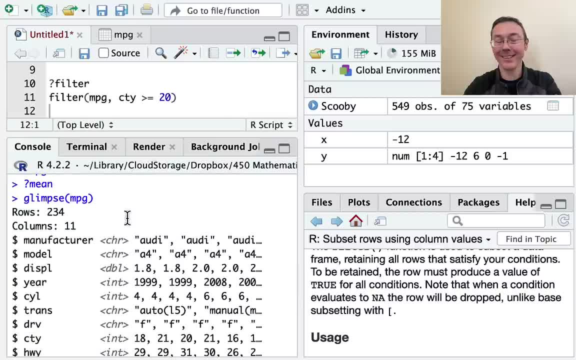 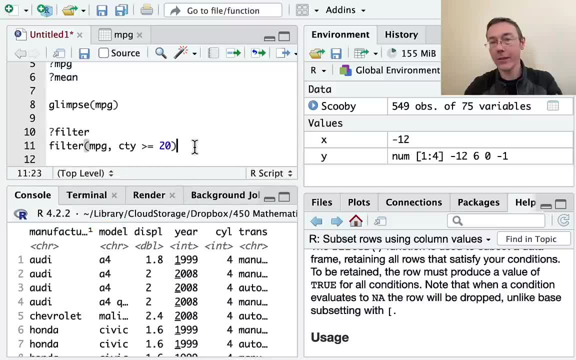 Many, many more than I had before. If I go up and look at that glimpse command, I can see I had 234.. What I would really like to do is to take this command, make this filtered set, save it as a new value. 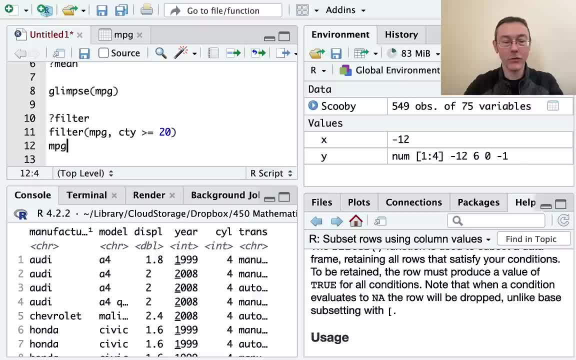 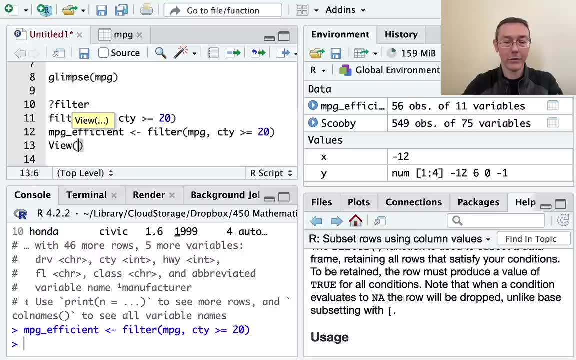 So maybe how about mpg efficient And then be able to do operations with that? So I'm gonna copy and paste, For instance, just right off the bat: maybe I want to view that mpg efficient. And now here in my viewer, I can see: 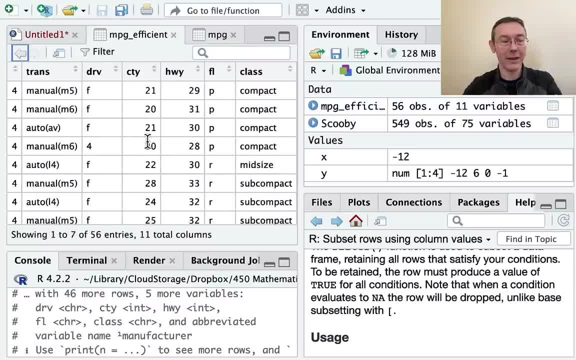 I can see that mpg efficient. And now, here in my viewer, I can see that mpg efficient. And now, here in my viewer, I can see that mpg efficient. That all these cars have city mileage of at least 20.. That all these cars have city mileage of at least 20.. 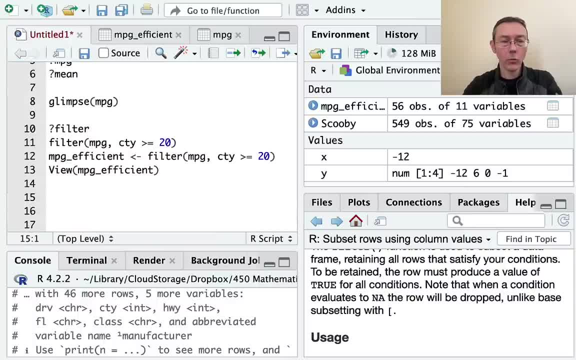 That all these cars have city mileage of at least 20.. Great, Let's do one more filter. Let's take a mpg, let's call this Ford And let's do a filter. So that was that manufacturer? I think Yes, manufacturer. 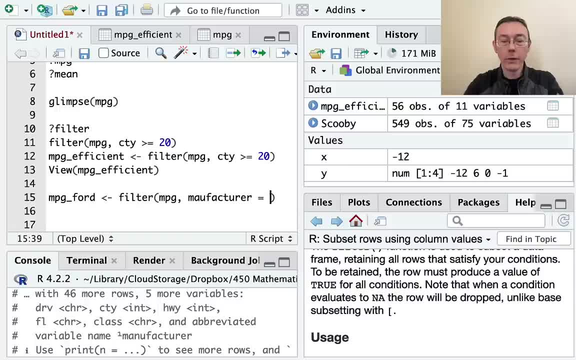 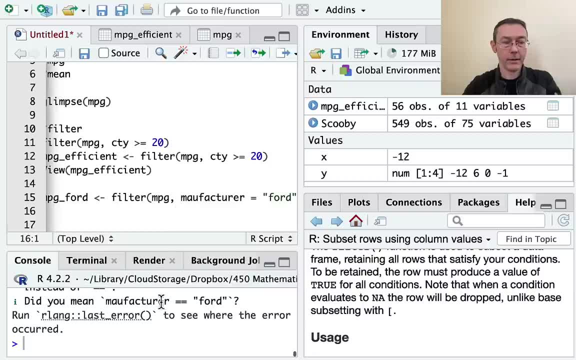 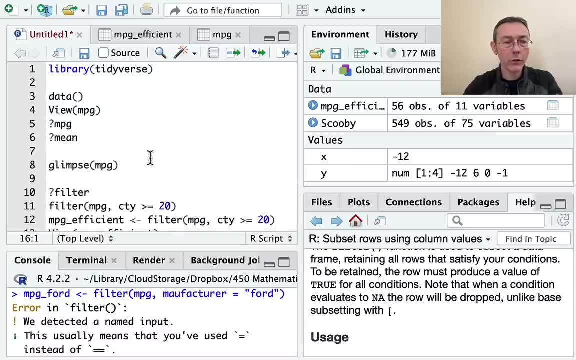 should be quote forward Now. if I hit Command-Enter right now I'm going to get an error. We detected a named input, So remember when I was doing an optional argument on that mean command earlier, which was pretty far back. 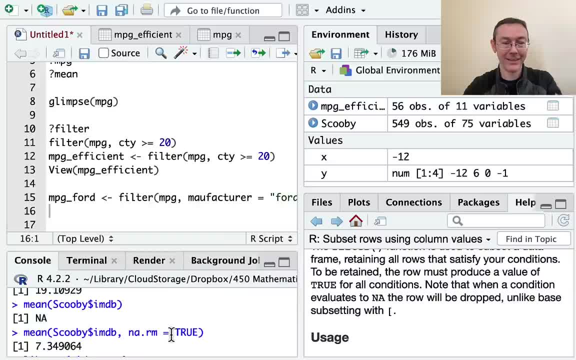 Let's see here. Should I even try and find it? It's up here somewhere. Yes, I named the argument. narm equals, true. So here r is looking for an argument called manufacturer. That's not what I mean. I mean I want a value of a variable. 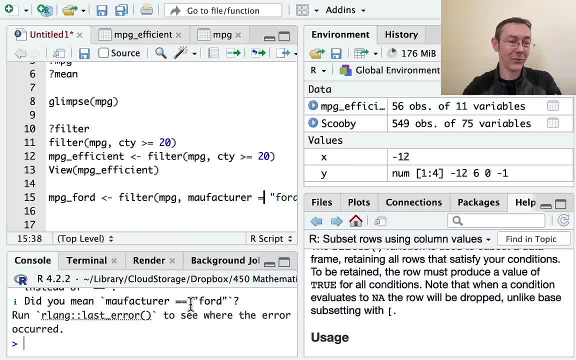 So the equal sign here that I'm looking for is actually different than the equal sign that r thinks I mean To specify this kind of logical equality that I'm looking for. I want a double equal sign, And now that'll work, And I misspelled it. 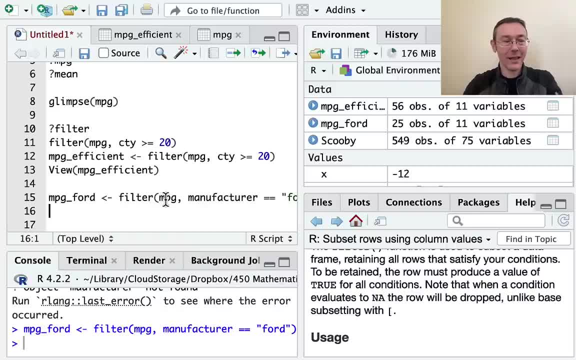 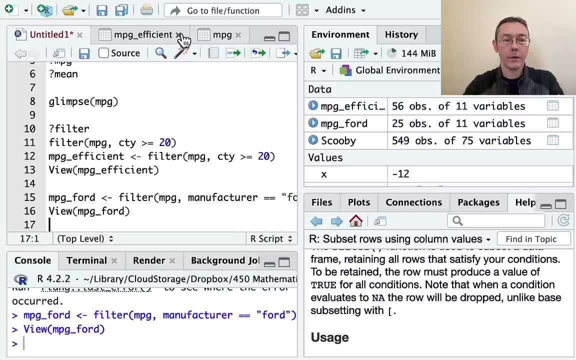 Manufacturer. Now it will actually work. And let's just take a view of that mpg underscore forward. There it is And you can see now it's all forwards. Great Neaten- that up a little bit, I think. the next most common data task. 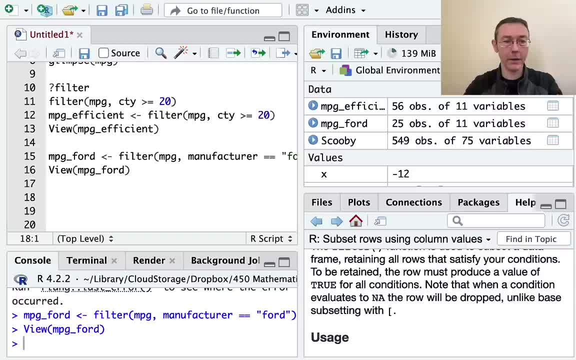 that you might have is to add or change a column in a data set, So I'm going to do. One of the things I notice in this set is that the units of measure are metric, I'm sorry, are standard Miles per gallon. 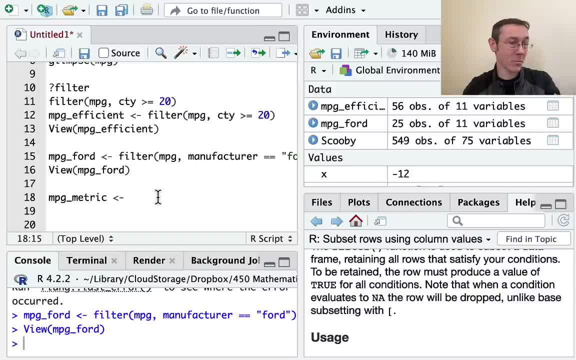 And I know many people in my audience will be unfamiliar or less comfortable with miles per gallon than, for instance, kilometers per liter. So let's take the mpg data set and add in a new column that is going to have the city mileage in that new unit of measure. 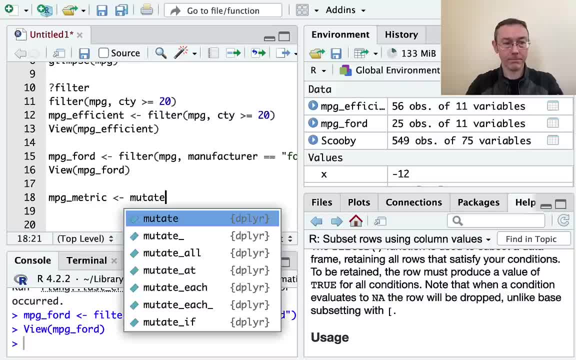 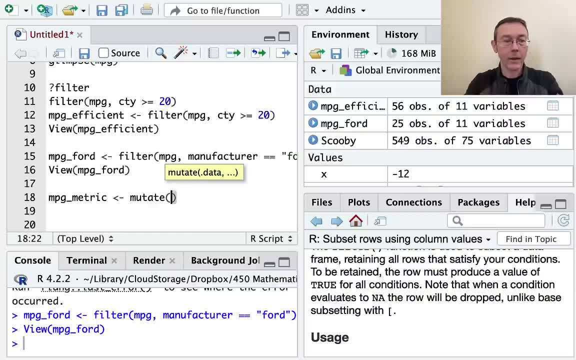 The command I'm looking for is mutate, And mutate is going to add or change a variable in my data set. As with filter, the first argument should be the name of the data set, And then after that I need to specify the name of the column. 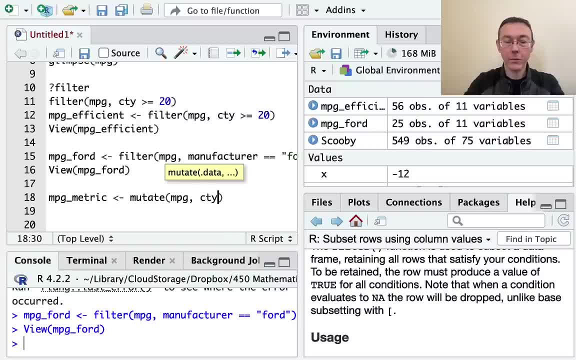 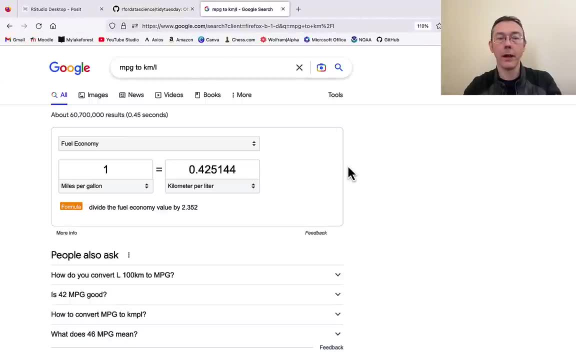 that I want to add or change. So in this case it's going to be cty metric And I need to specify a formula for this new column. So I googled the conversion factor for converting miles per gallon to kilometers per liter. 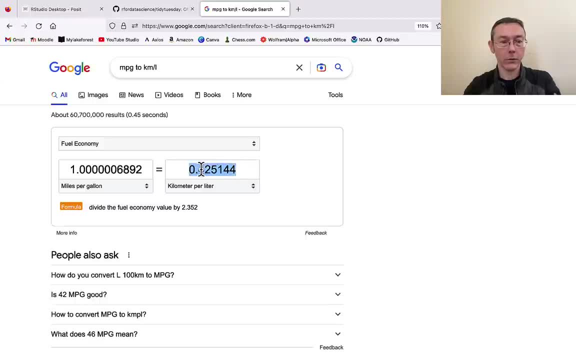 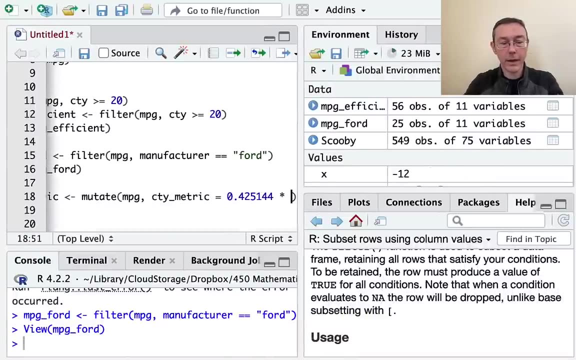 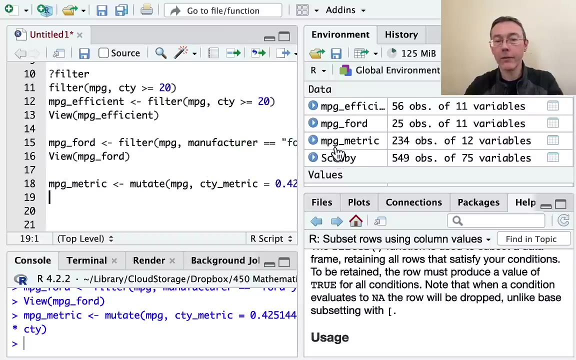 And it is this number right here, So let me just copy and paste that. So I'm going to do that. times the city mileage. that was in miles per gallon. Command enter And you can see. I now have a data set called mpg metric. 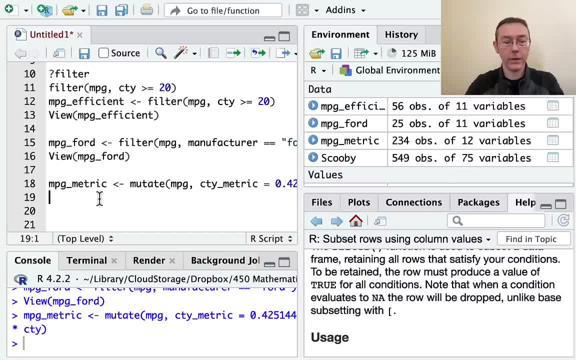 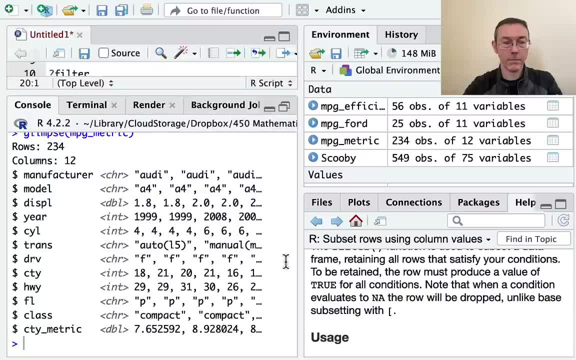 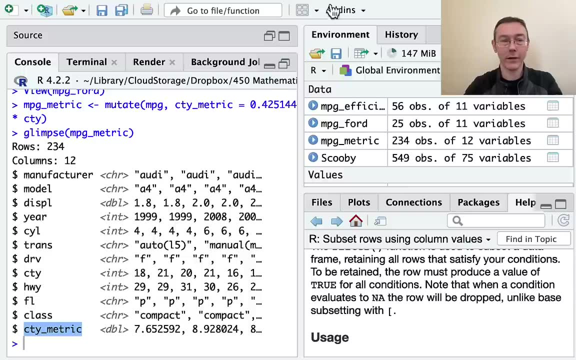 Instead of having 11 variables, it now has 12., And maybe I'll glimpse this. Okay, All the same, until I get to this last column, there is a new column called city metric, just like, I would hope, Another very, very important thing in R. 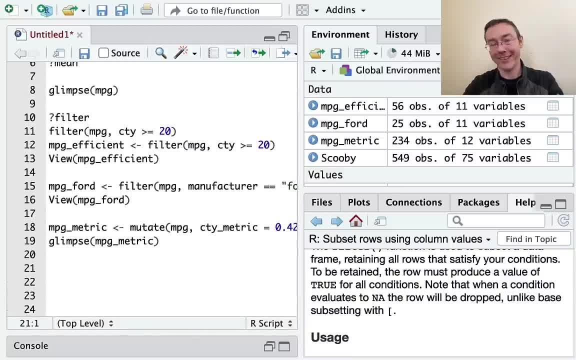 is- let me start that sentence again. Frequently in R you'll be doing long procedures where you start with a data set and do a number of different things to it: First filter it, then add a new column, then maybe do something else. 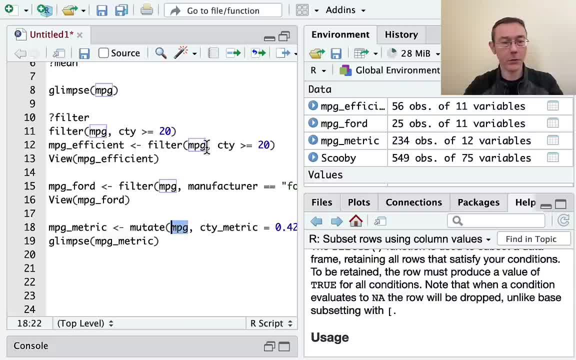 And we have this standard syntax among many, many verbs in R and in particular in all the tidyverse verbs where the first argument is just the data set, And you'll find yourself doing verb parenthesis, mpg, over and over and over again. 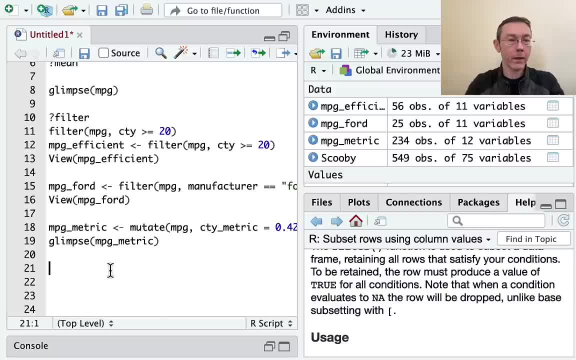 And that gets inconvenient for any number of reasons, And so there's actually a tool built into R to help you get around that, And it's called the pipe, And the pipe just takes an argument and passes it to the next function as the first argument. 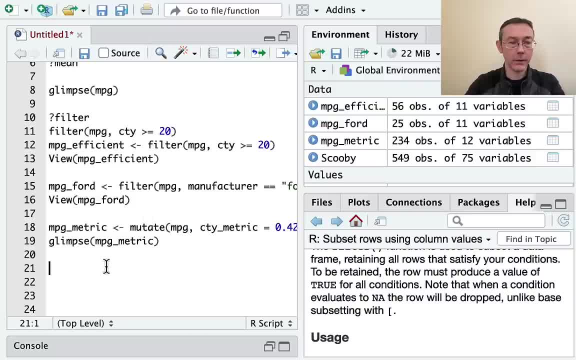 So I'm going to redo this mutate command using the pipe. So it's still mpg metric. That's still the output I want. But instead of putting mutate mpg, I'm going to put mpg pipe mutate And I'll start a new line. 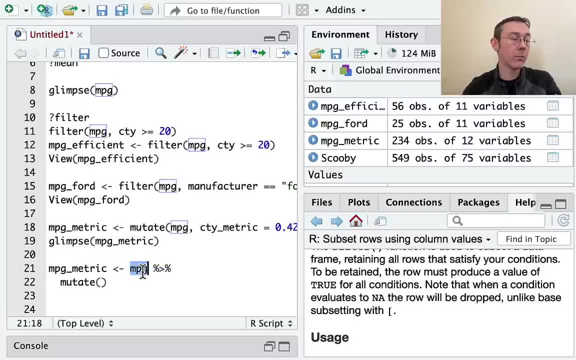 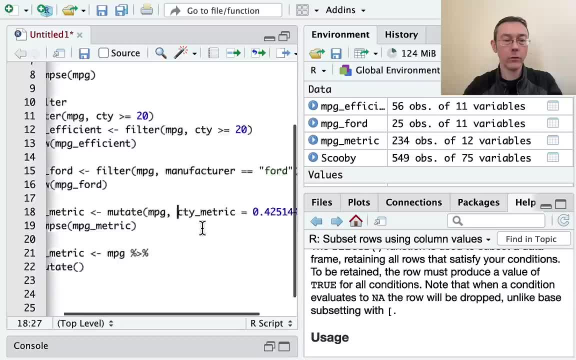 so it's a little bit more neat. What this is saying is: take the mpg data set and pass it as the first argument into the mutate command. So now all I have to do is put in this conversion the second part of it. 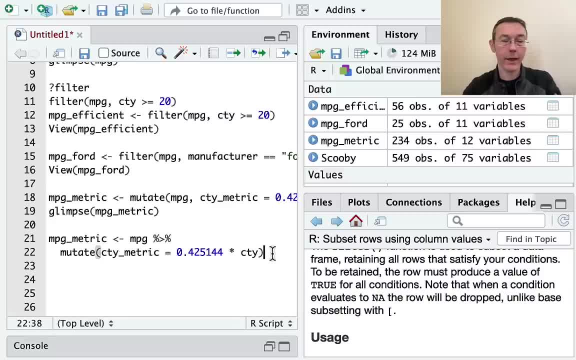 And then if I wanted to do another argument, another function after that, I could do another pipe, for instance, and then a filter command or whatever. This becomes very natural to read in English or whatever language you happen to be speaking, just from left to right. 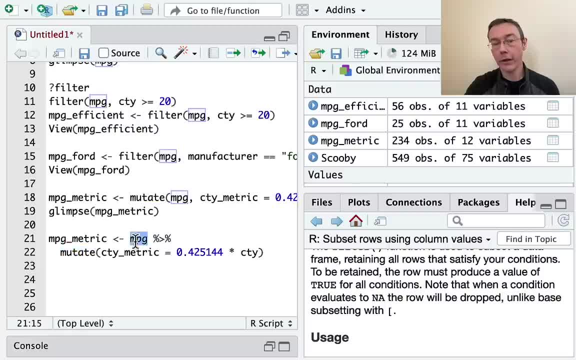 because it's noun and then verb. So take the mpg data set and mutate it in such and such a way, And if there were another pipe here, I'd say and then, and if there were another verb here, filter it or whatever else you might like. 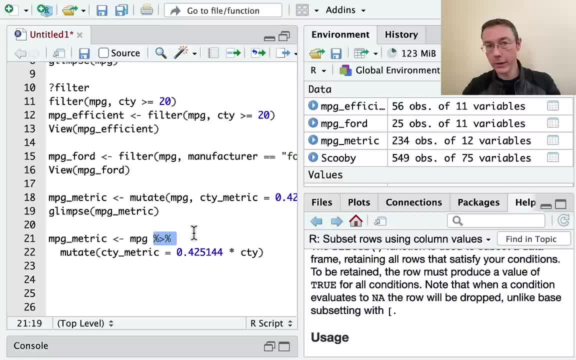 By the way, there's a keyboard shortcut in R for this pipe. You saw that I didn't actually type the characters one by one. It is command shift M on a Mac or control shift M on a PC, And you will use that shortcut. 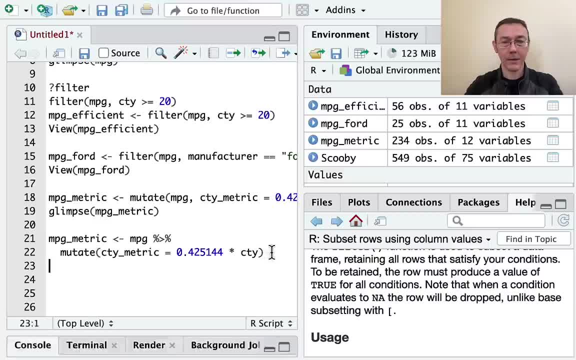 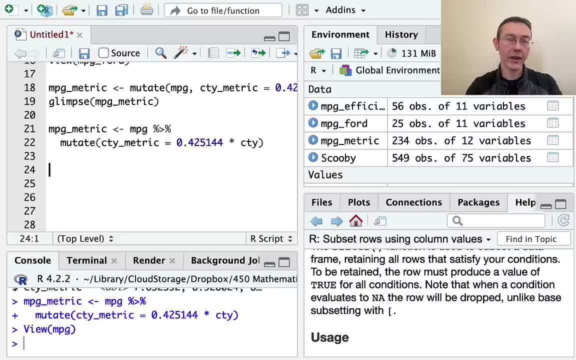 more than probably any other keyboard shortcut. So you can use that shortcut when you're using R, And so if I execute that, the same thing happens as did before. Another hugely common data analysis task is to get grouped summaries. So, for instance, 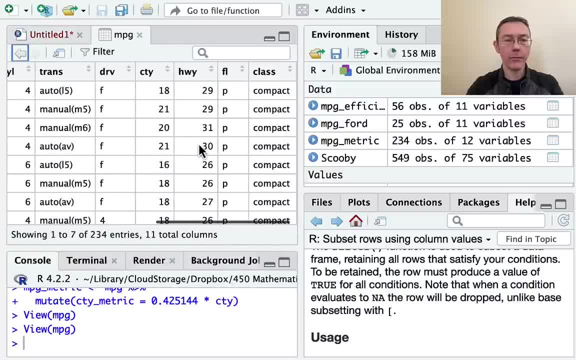 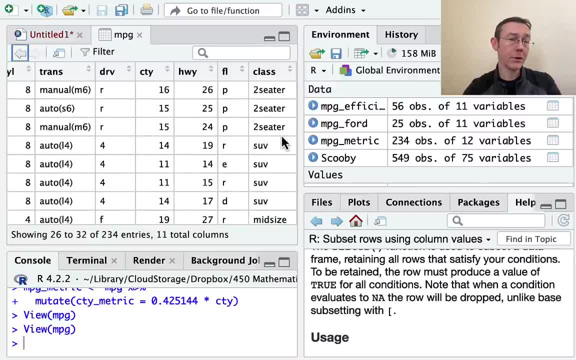 let's take a look at this data set one more time. We have several different classes of vehicles- compact, midsize, two-seater SUV and so on- And I might want to know how is the average city mileage different in these different classes? 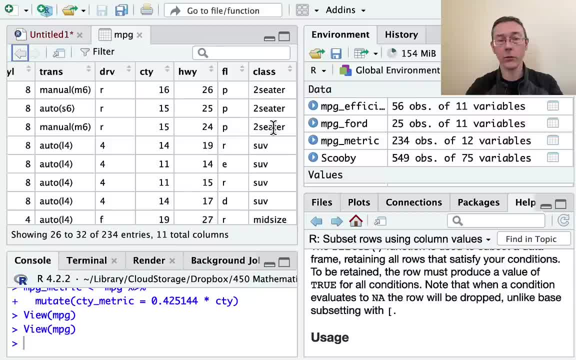 Now there's a bunch of different classes, so it's not really so convenient to do a filter over and over and over again, followed by a mean. We'd like to automate this process And R and the tidyverse family packages, in particular, have a very natural way. 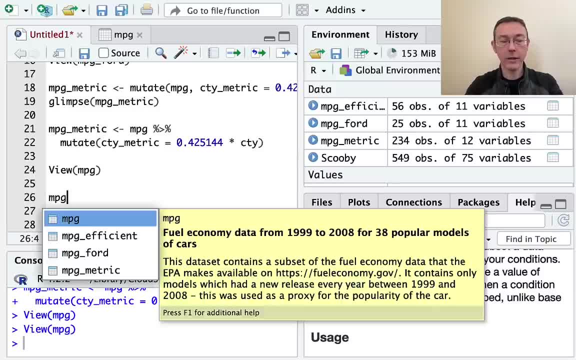 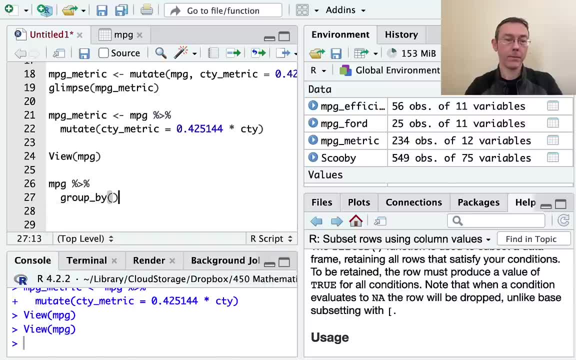 of doing that. So I'm going to take the MPG data set and, using my new pipe operator, I'm going to pass that as the first argument into this group by command And group by is just literally going to take this data set and view it now as grouped. 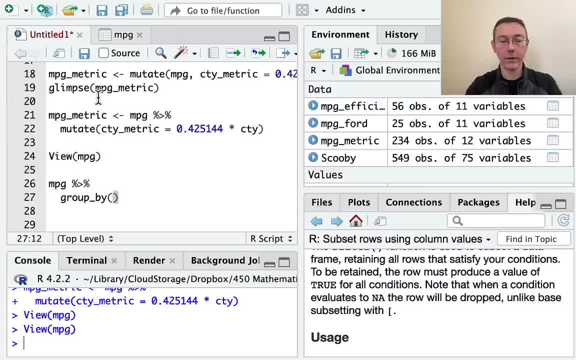 by whatever categorical variable I might pass it. So in this case I want to group it by class, And after I've grouped it by class I'll do another pipe. So I'll take that data set and pass it in to a summarize command. 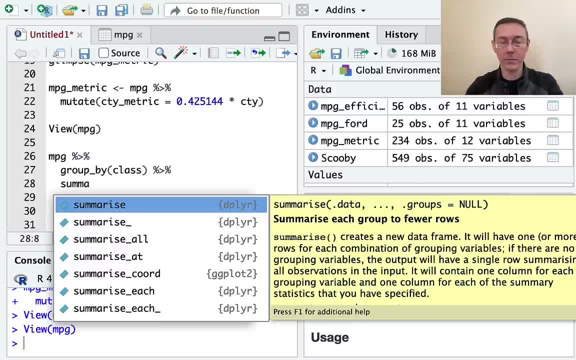 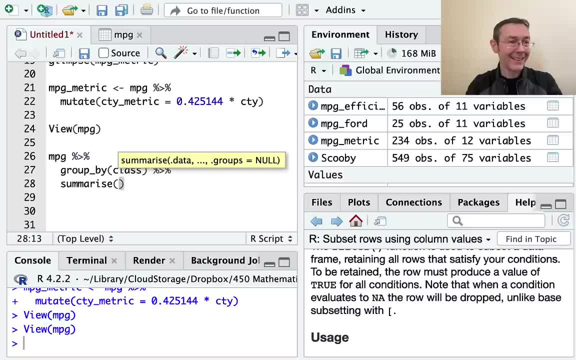 And you can use an S or an E. This was originally developed, I believe, in New Zealand, So S is the default, but Z will work if you're in the United States, for instance. So now it's grouped by class. 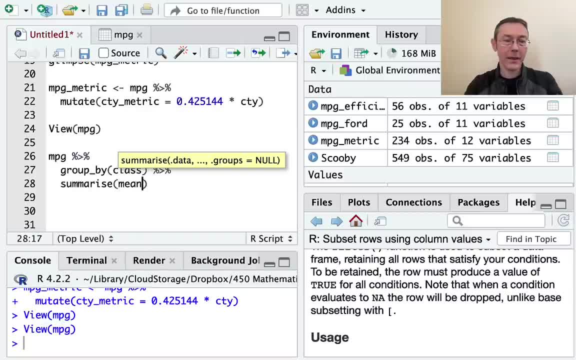 I have to say what operation I'd actually like to perform And I'd like to take the mean of the city mileage. So I'll execute that. This is going to take the MPG data, set group it by class and then take the group means. 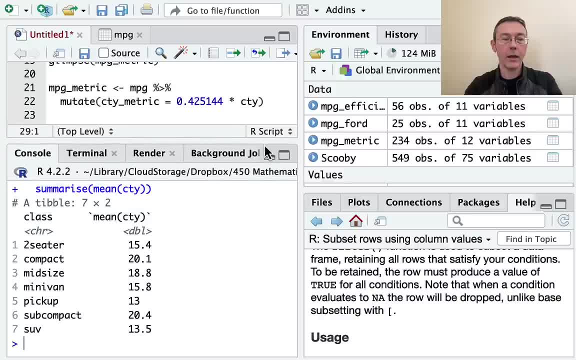 When I command enter, that the whole thing will be executed And I get a data set back. In this case it has seven rows. I get the average mileage for the two-seaters, the compacts and so on all at once. 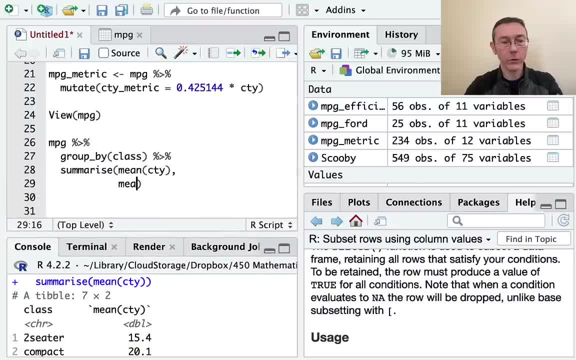 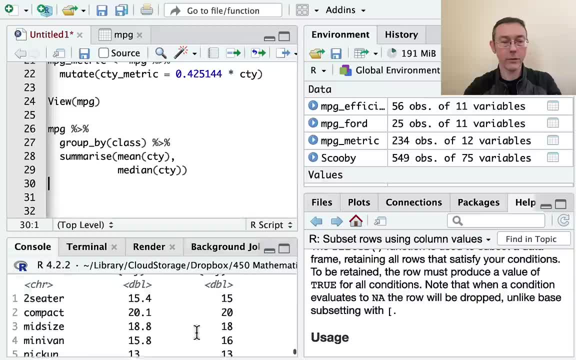 And I can do that. I can do more than one thing at once. For instance, suppose I also want the median of the city mileage. I'm just going to put both of those in And you can see out. I now got an extra column with the medians. 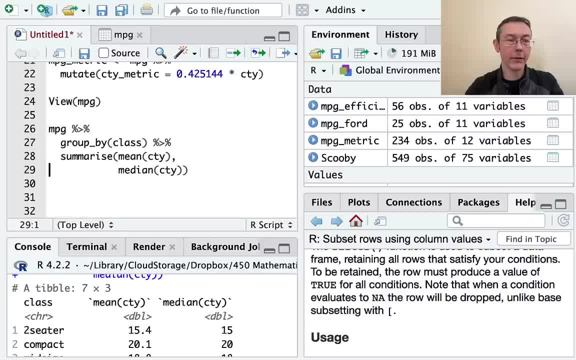 I should talk about these line breaks here. Notice that I've been sometimes hitting enter at the end of a line and getting this indenting If you hit enter after a pipe or a comma or another place where R is expecting more in its command. 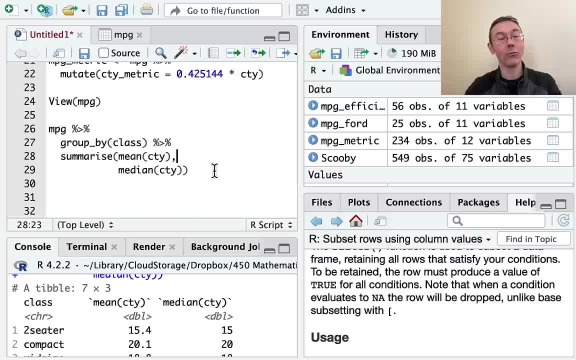 it will indent things for you. RStudio will indent things for you and recognize that you're intending to carry on the command on the next line, And that can be really helpful when you get these longer commands. This is much more human readable than it would be. 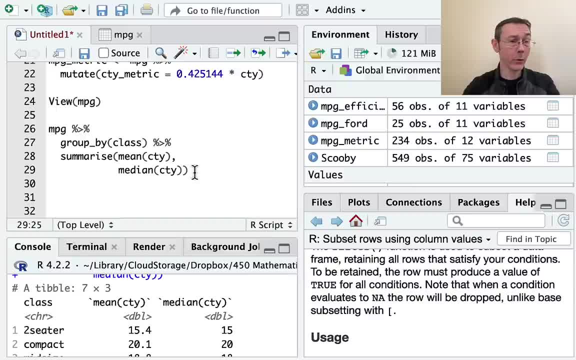 if I'd put this all on the same line. There are entire style guides devoted to the best way to indent your code, And as you get deeper into this, eventually you'll need to make a foray into that. Okay, we have two more things to accomplish. 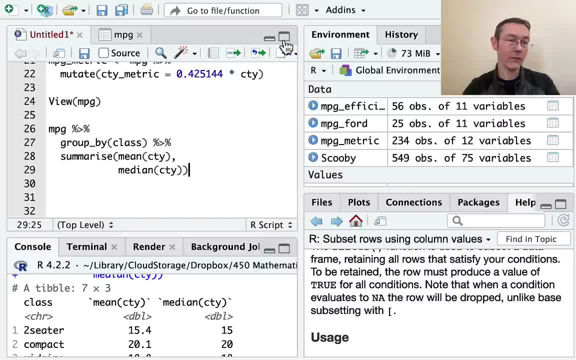 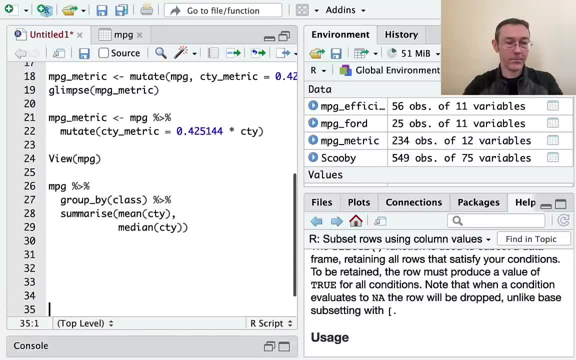 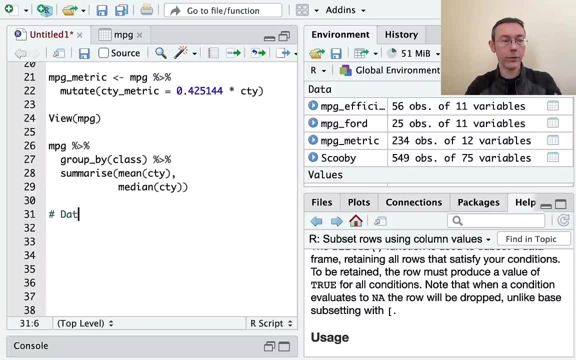 First of all, a tiny little bit of data visualization And then, second of all, a little bit about communicating your results. I think before I start visualizing, let me mention that you can insert comments into your code with a hash. So this lets R know that. this next line. 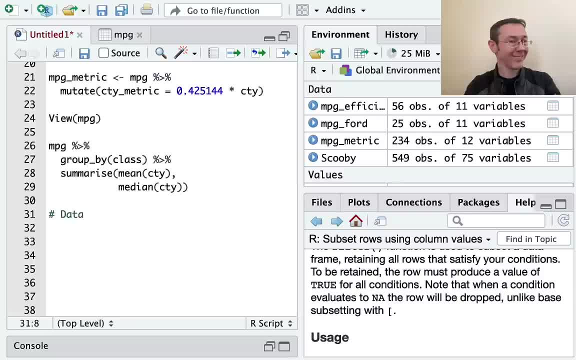 the next thing I'm going to write. this isn't actually code. This is supposed to be a comment for a human reader, So I'm going to do a little data viz. There's lots of different graphing systems in R- By far the predominant one. 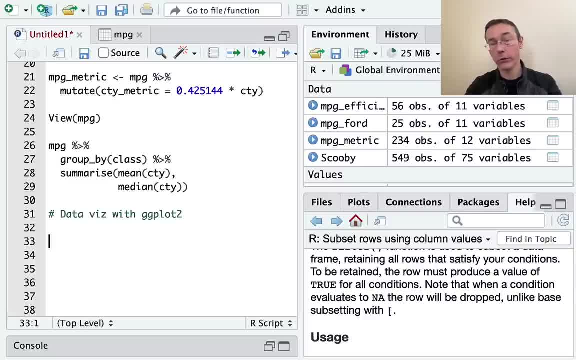 by far the standard one these days is ggplot2.. And so I strongly recommend that you use that rather than the base plotting package or anything else. This is part of the tidyverse. The ggplot2 package is one of the core pieces. 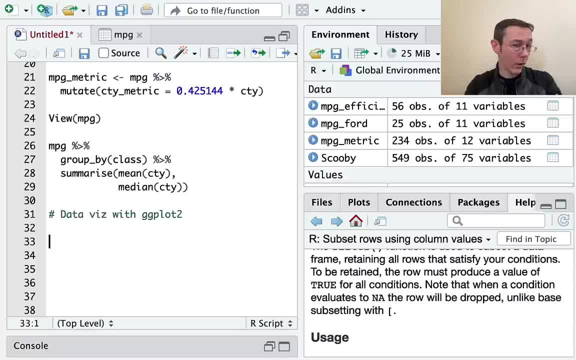 of the tidyverse. gg stands for grammar of graphics, And it's a rather revolutionary idea. I think that when you look at a data visualization, there are some very key components that are common to every data visualization, And so when you're specifying a plot, 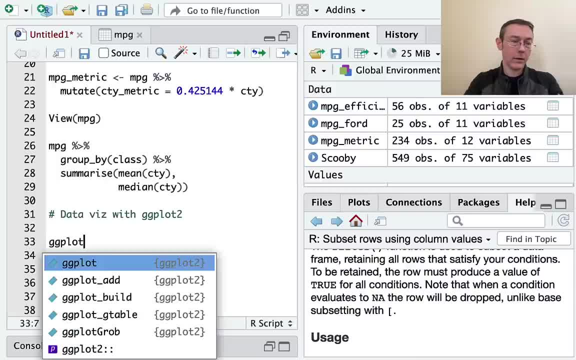 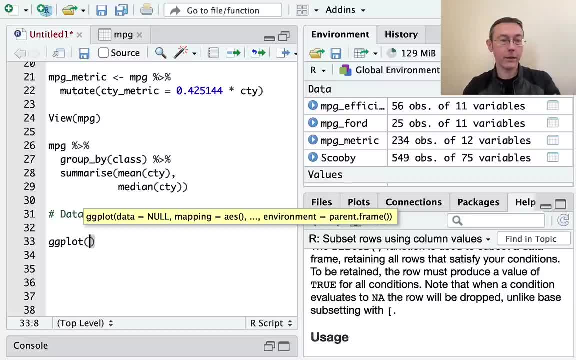 you should follow that fundamental structure. That'll be clearer as I do an example. So in R, in the tidyverse family of packages and ggplot in particular, we have one workhorse plotting command, not one command for every sort of plot like you would in some languages. 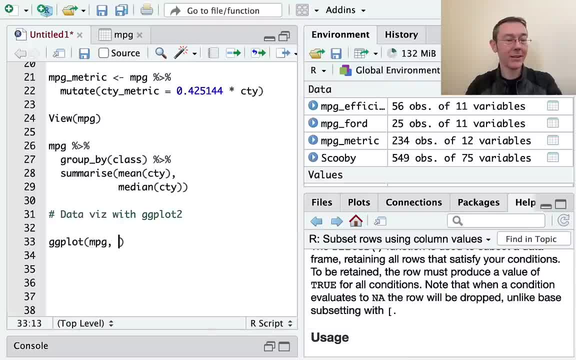 ggplot. First we specify the name of the data set. Our assumption in R is that we're working with data. The philosophy behind the grammar of graphics is that the fundamental thing about a plot isn't so much whether it's a histogram or a frequency polygon or a scatter plot. 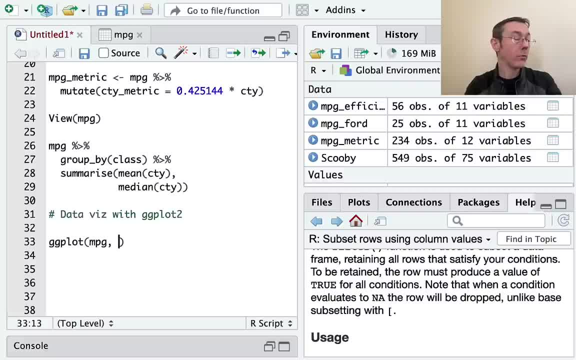 but rather what variables are being communicated in which ways On the x-axis, on the y-axis, with color and so on. So we're going to specify which variables are being communicated in which ways first, and only later specify the sort of plot we want. 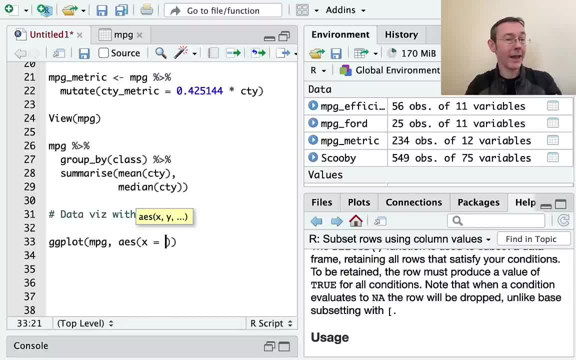 So in this case I want to specify an x-aesthetic. On the x-axis of my plot, I'm going to want city mileage. So aesthetic is just the way of saying what variables are going to be communicated in which way. If I execute this command right now, 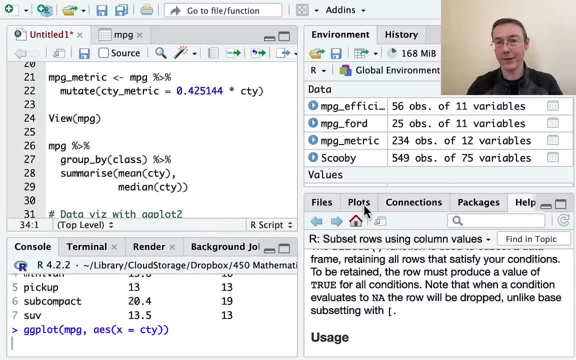 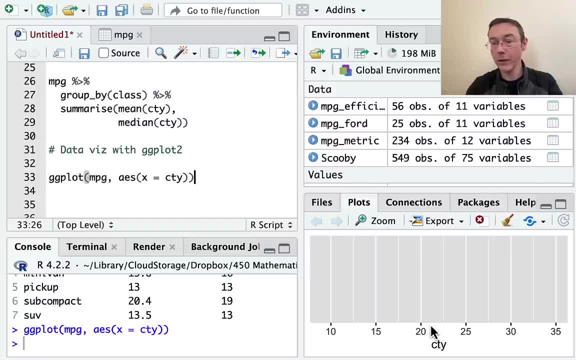 something will come up in my plot pane in a second. Sorry, I have an old computer and it's going slowly, But it's not very interesting. You can see it's put city mileage on the x-axis but not actually plotted any data. 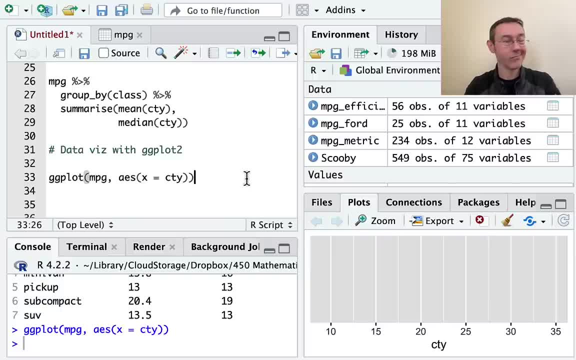 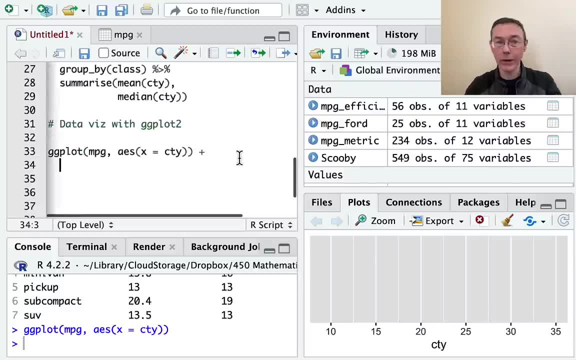 And that's because I haven't actually specified what sort of plot I want, so R doesn't know how to actually visualize that. I'm going to put a plus and then, to make it read a little better, I'll start a new line. 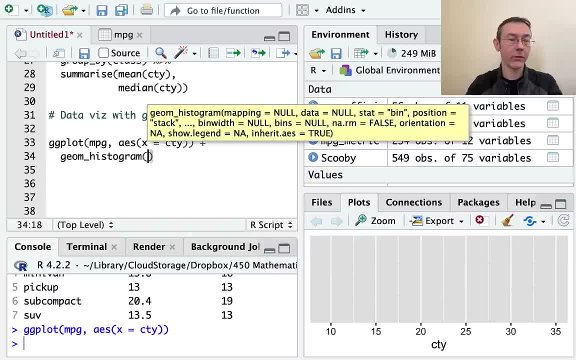 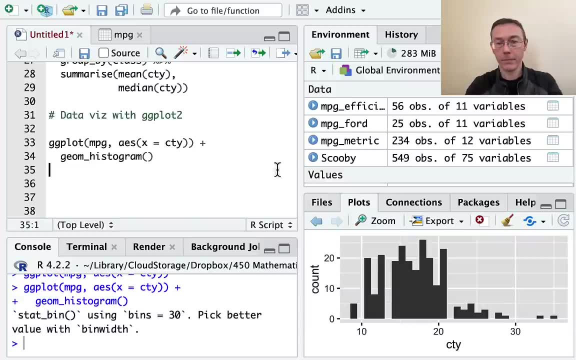 and then actually specify the sort of plot I want And the syntax for that is geom, underscore, and then the type of plot. So in this case, let's get a histogram. There we are. There's a handy little zoom button. I'll click that. 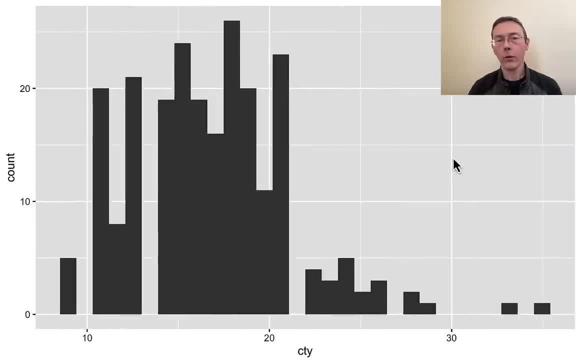 There, it is Okay. So there's any number of things we could do to make this plot look nicer. We could change the labels, We could put a title on it, We could change some colors, Lots of different stuff. I'm not going to get into that in depth. 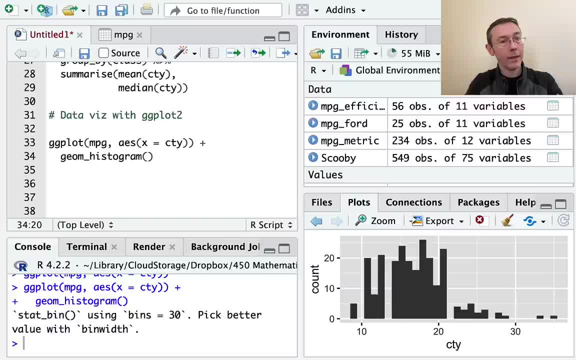 except to say that the grammar of graphics is layered, and the idea is that we should first get the basic plot and then go back and change the non-data aspects later, for instance with plus labs, And for instance we can change the x label. 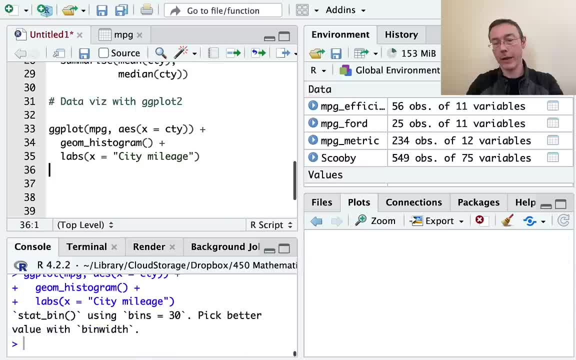 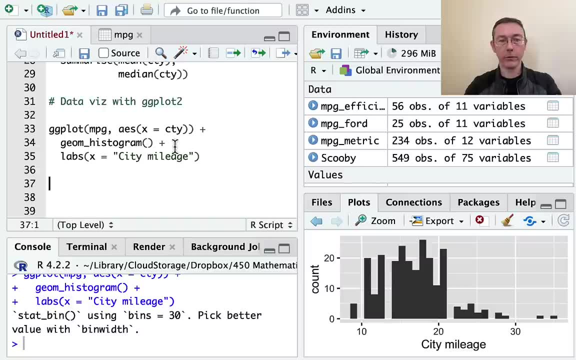 to be city mileage, And when I execute that, you'll see it's changed. the x-axis label: Okay. So this seems rather verbose. Why should we bother with all of this when we could just have a command that said histogram? Well, one reason. 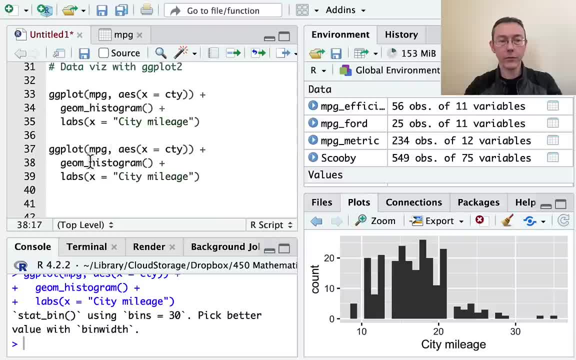 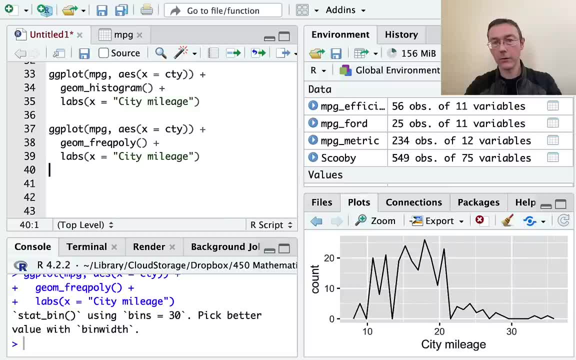 is that there's not really anything different between this plot and, for instance, a frequency polygon, And if I execute this command, you'll see the plot looks fundamentally the same, even though it's no longer a histogram. The key point to both of these plots- 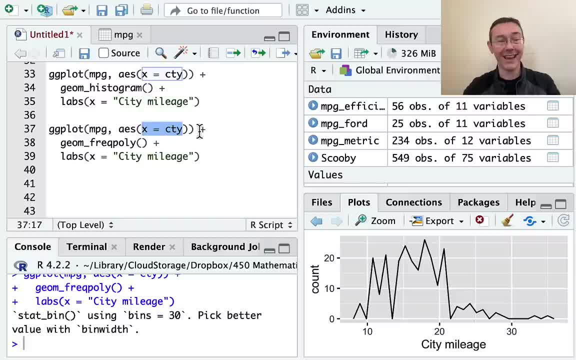 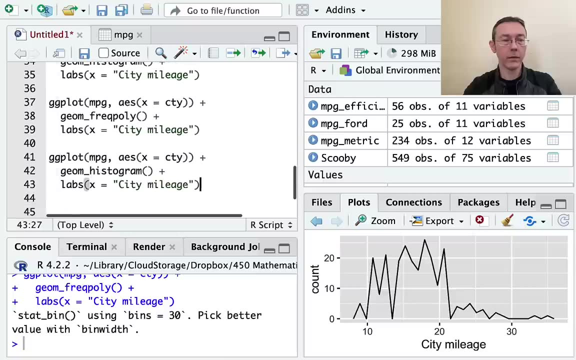 is that city mileage is being put on the x-axis. The fact that the one is a frequency polygon and the other is a histogram really is secondary. This becomes really difficult and really powerful, for instance because- and I'll just copy and paste again- 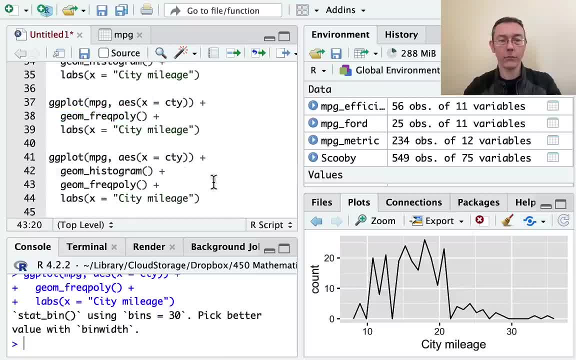 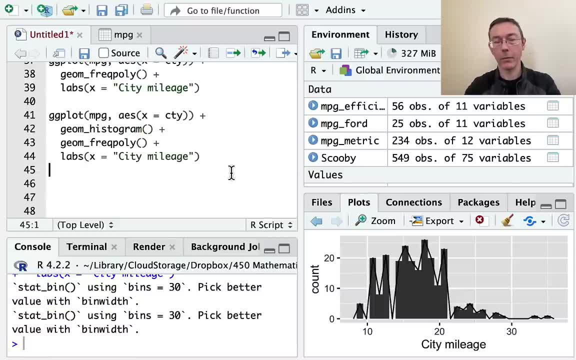 we can actually do both at once, So I'll do a histogram and a frequency polygon at the same time, And this isn't maybe the best plot, but it illustrates an important point. Once that comes up, you can just layer things on however you want. 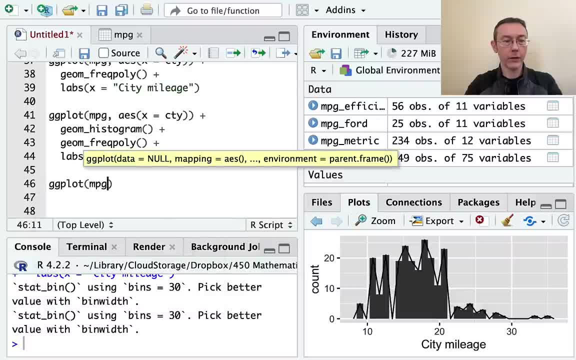 Let's do just a couple more plots with the mpg dataset. Let's get a scatter plot, City. Let's also get a y-aesthetic this time. Let's get highway mileage. So city versus highway mileage Makes sense. Obviously, I don't want a histogram anymore. 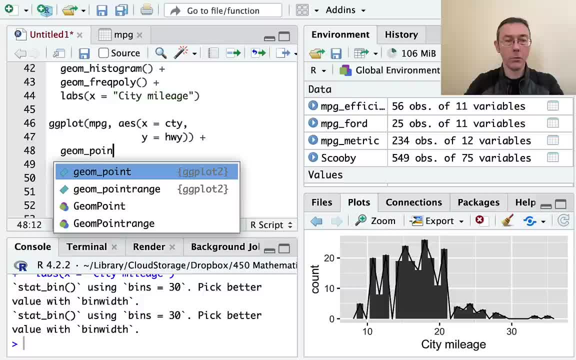 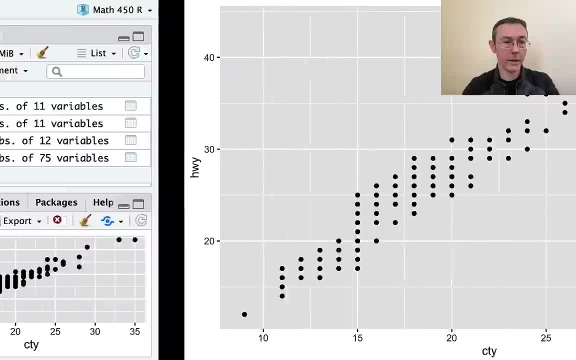 I want a scatter plot, So let's do that with geome. So this is how I get a fundamental scatter plot using ggplot, And I'll zoom in on that. You can see city mileage on the x-axis, highway mileage on the y-axis. 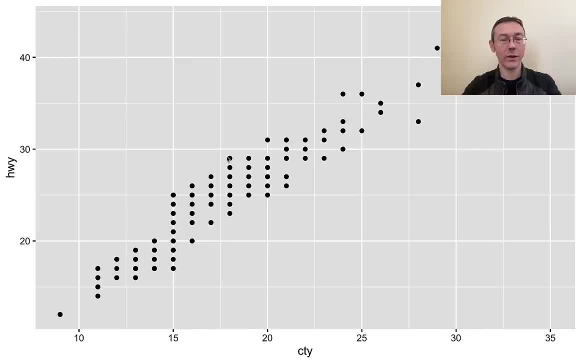 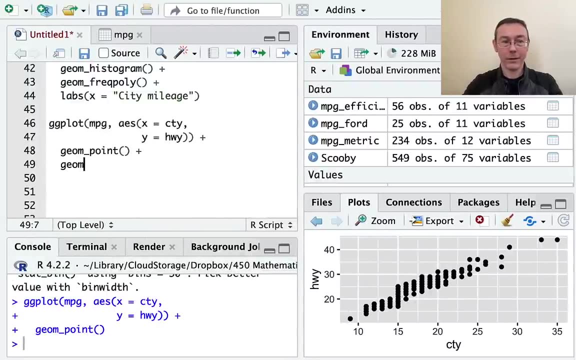 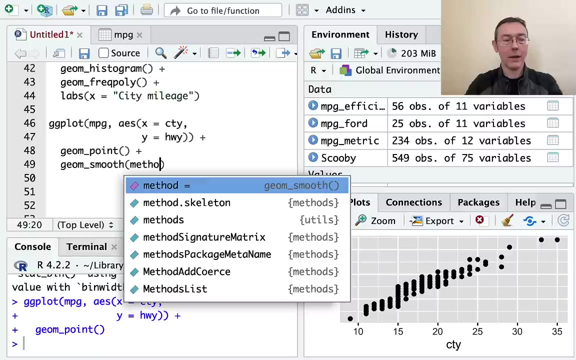 Not surprisingly, there's a fairly linear relationship between those two. Oh, linear relationship. Let's put on a regression line, Another layer, Geome smooth. There's many different ways of putting smoothers on top of plots. I want a linear one. 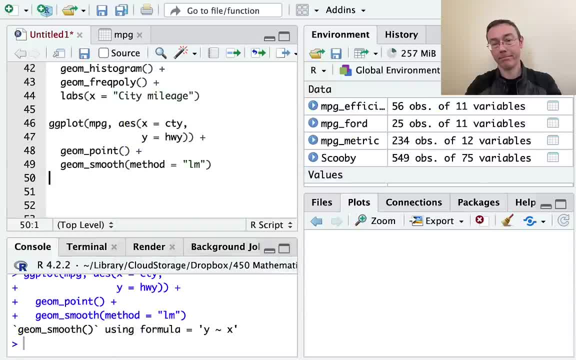 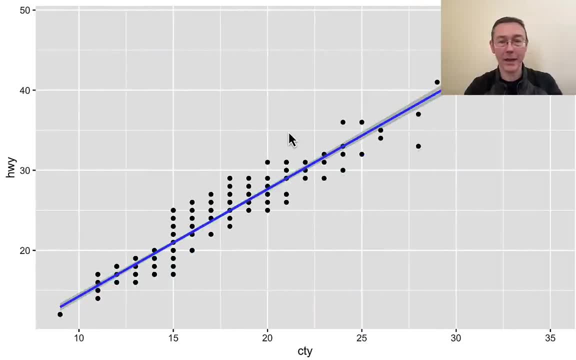 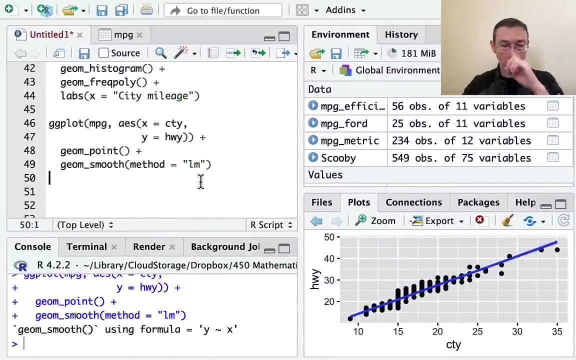 The syntax for that method equals lm, And there's my regression line. You can see a little gray band here. That is a confidence band. So, um, I won't talk too much about this, about that, right now. Let's see here: 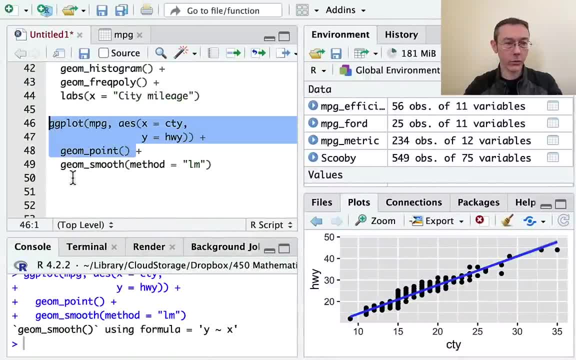 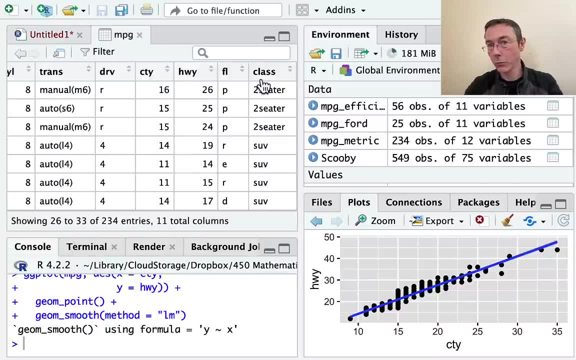 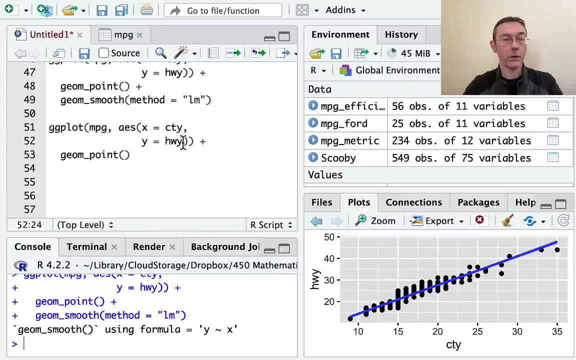 One more thing with this scatter plot that I'd like to show. I'll leave out the regression line for now. Remember, I have different classes here. I did some group summaries with those earlier. I want to show how to get different colors for the different classes. 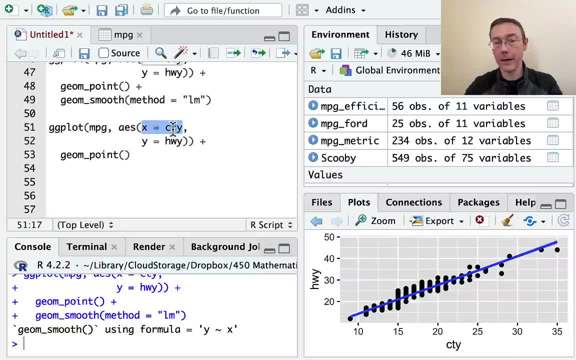 So, just as the city mileage is being displayed on the x-axis and highway mileage is being displayed on the y-axis, I want to add another aesthetic here, saying how the class variable should be displayed. Now, I don't want that on an axis, I want that to be displayed with color. 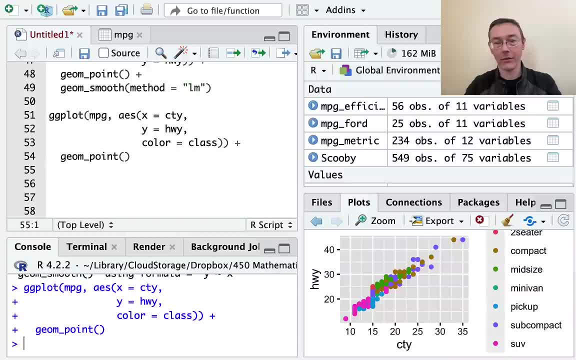 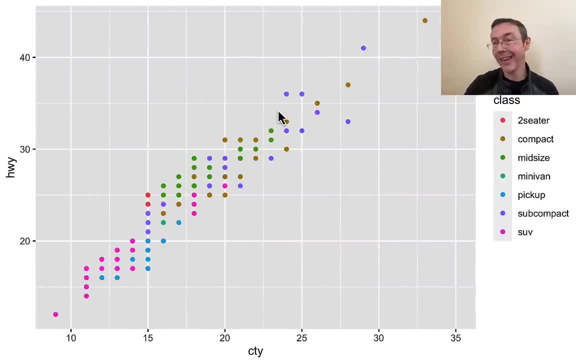 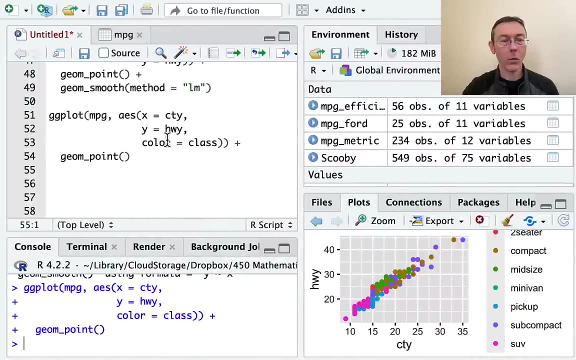 So I'm just going to add an extra aesthetic And I'll command enter on that. Okay, So now each of these points has a different color and there's a key on the right letting you know which color is representing what class. Now, just as we can layer different labels, 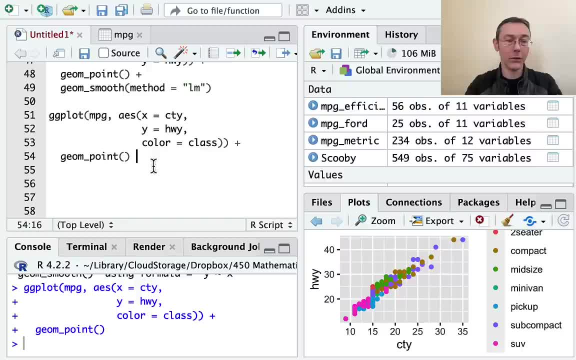 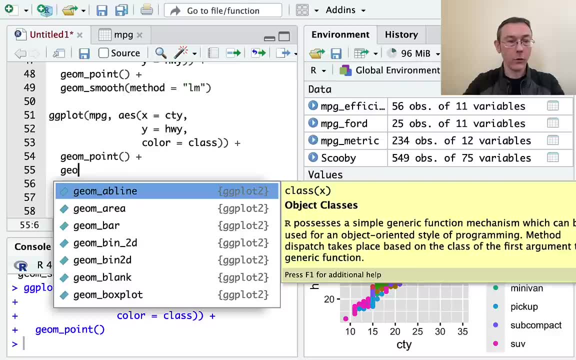 we can also change the colors that are actually being used here. You can do that by hand, But what I recommend is that you choose a built-in color palette. So that's not a geom. sorry, It's changing the color palette. 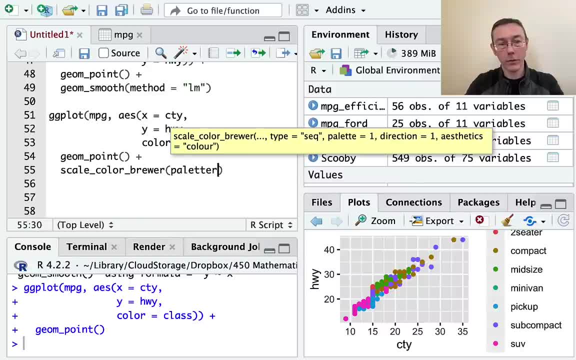 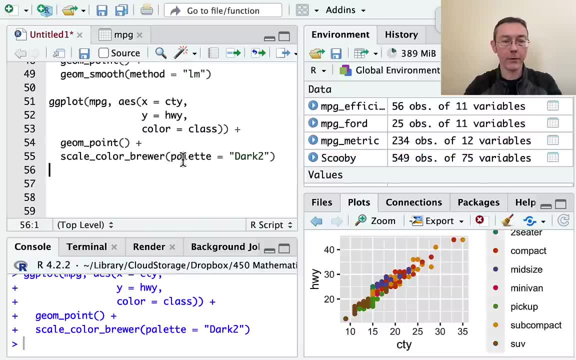 So scale color brewer And I'm going to use the palette that's called dark2.. And I like this one because it's color blind friendly, Unlike the base palette. There we go, So that looks a little better. I want to close by talking. 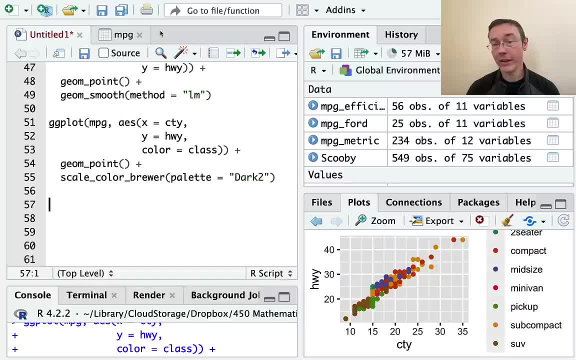 a little bit about communication of results. As your data science skills improve, you're going to want to share your results, either with supervisors in your jobs or with clients, or just with friends, And it's awkward to be writing word documents and dragging in visualizations like this one from R. 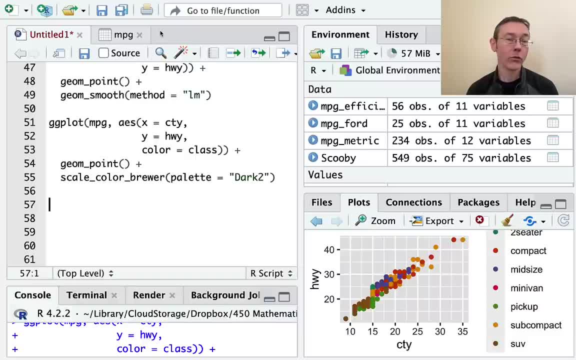 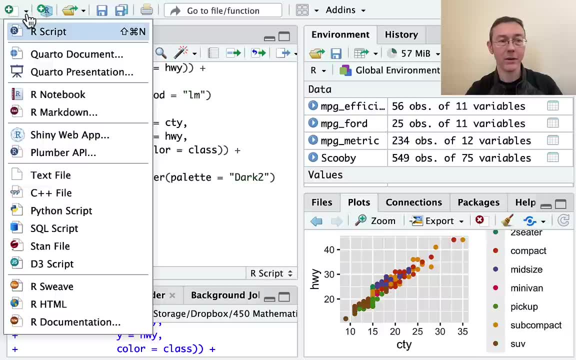 or copying and pasting tables. Fortunately, RStudio provides a great tool for this. It's the markdown document, So let's create one of those. I'm going up to the new file thing here And just going a little lower than R script. 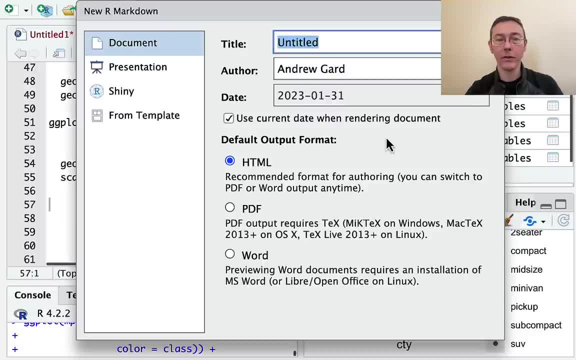 to R markdown. There's some various options here. I'm just going to leave them all as is. HTML is a good all-purpose format, both from RStudio's perspective, from the coding perspective, but also just in terms of flexibility If you generate an HTML document. 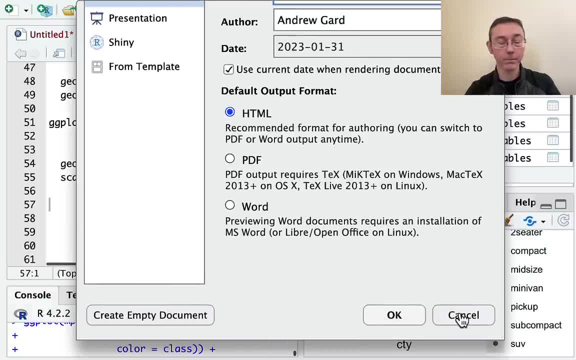 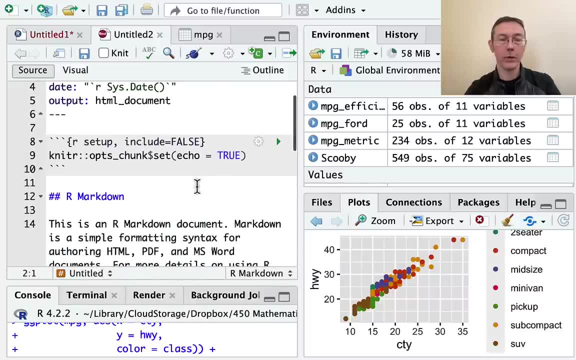 you can convert it to other things later using either R or other things, And when I open up that file, there's going to be a template that RStudio is going to pull up, And there's essentially three pieces to this. And, by the way, when you're starting, 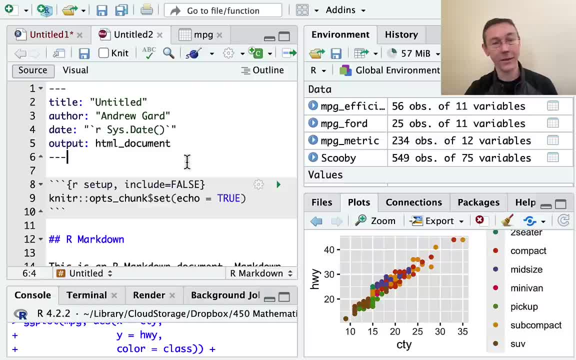 out and for a while after that. I recommend just modifying this template rather than starting from scratch every time. The first part of the document is this header, the so-called YAML header, And you can see title, author, date and output format. You can obviously modify. 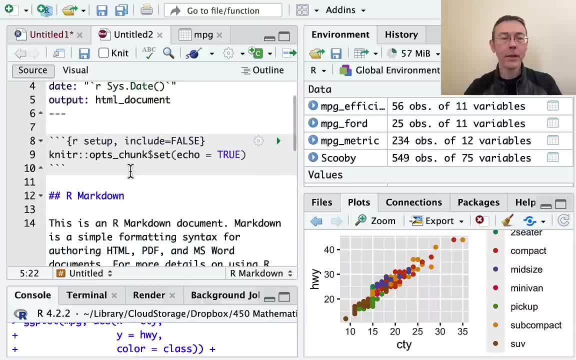 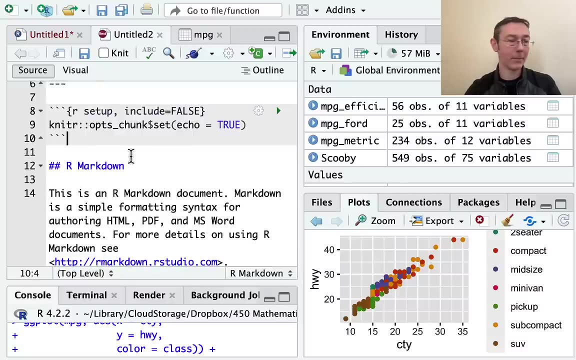 those first three as you see fit. You have these gray chunks with three hyphens or three single quotes before and after. This is R code, And so you can insert R code that the Markdown document will later execute if you want it to. Finally, 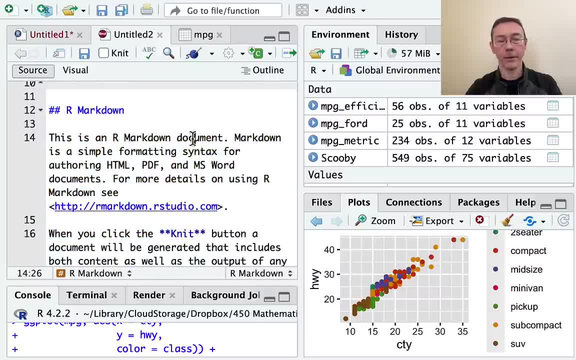 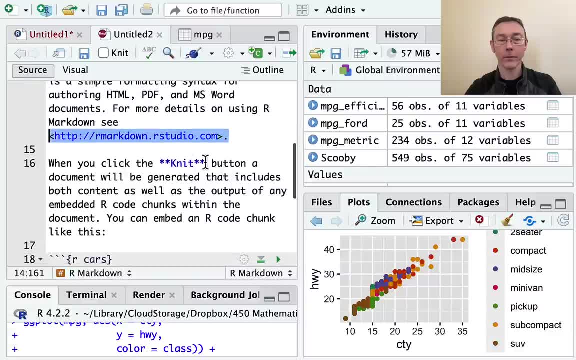 you have some lightly formatted text like: right here You can do headers- That's what's going on here- Links like this, And this is going to be boldface. There are some other formatting options as well. You can Google, for instance. 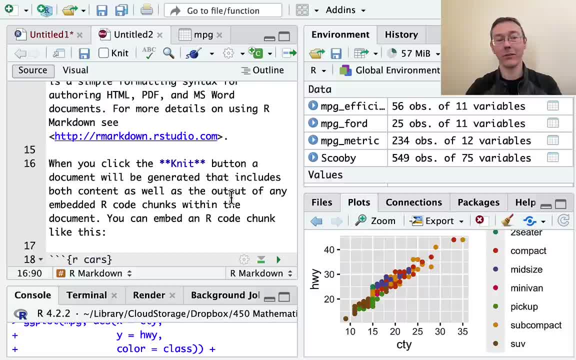 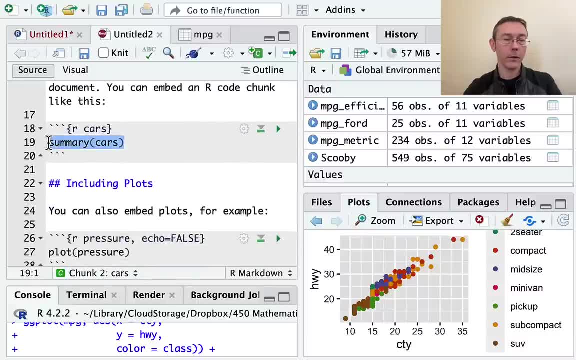 R Markdown Cheat Sheet to get some of the other commands at your disposal, And you can see that this template document includes some R code. So, for instance, let's change summary of cars, which gives some summary information about a built-in data set. 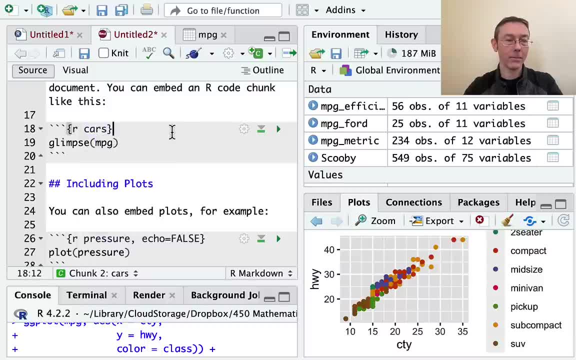 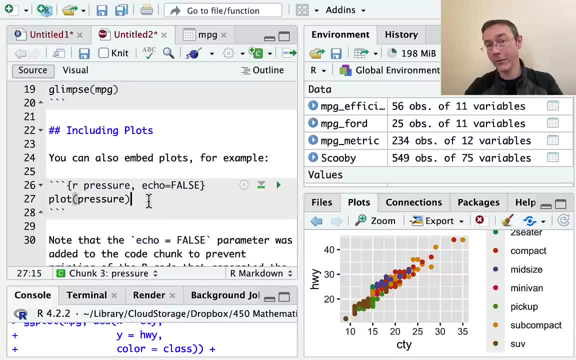 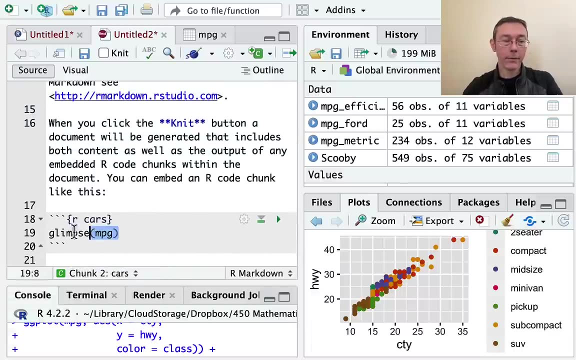 to a command we've already seen like glimpse mpg. Okay, You can embed plots. This is going to give a plot using the base R package. So when we see this plot it's going to be kind of ugly. Let's see here. 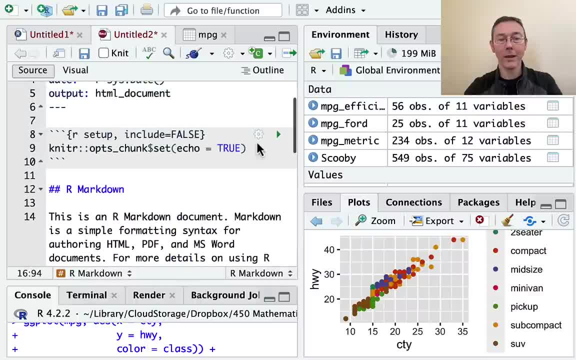 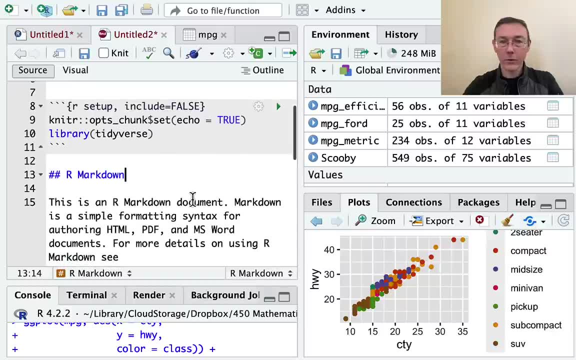 Remember that the glimpse command was in the dplyr package that was in Tidyverse. We've got to make sure that we load up Tidyverse. Let's do that. But, Dr Gard, didn't you already load up Tidyverse? 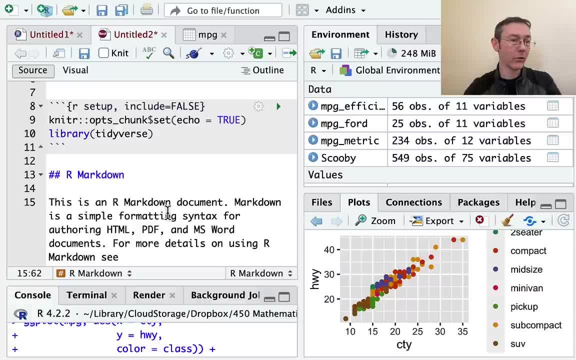 Well, when I go to actually make this code into a document, I've got to have something from a blank slate. So I've got to have things like library Tidyverse actually in the document. Okay, So I mentioned about rendering a document. 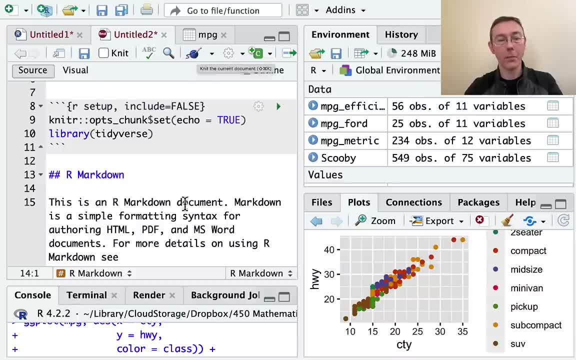 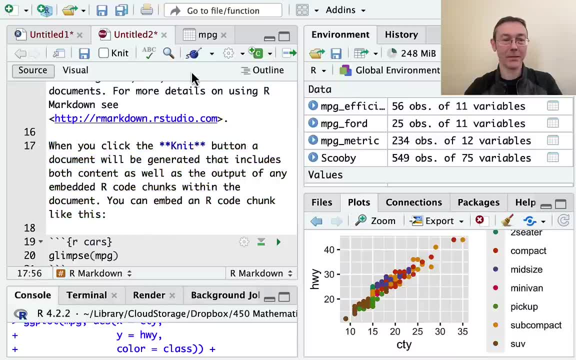 How do we do that? It's this little spool of thread here. It's the knit command And, by the way, that's actually written in the template document that you should click the knit button to actually generate the output. So let's see what happens. 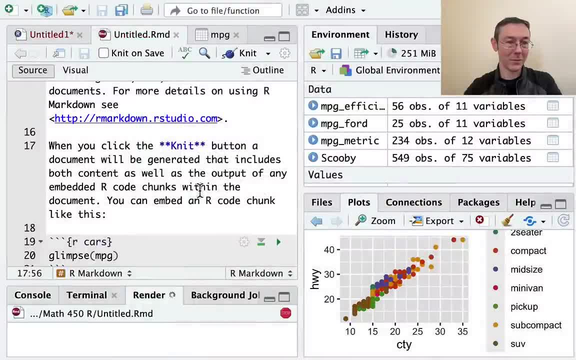 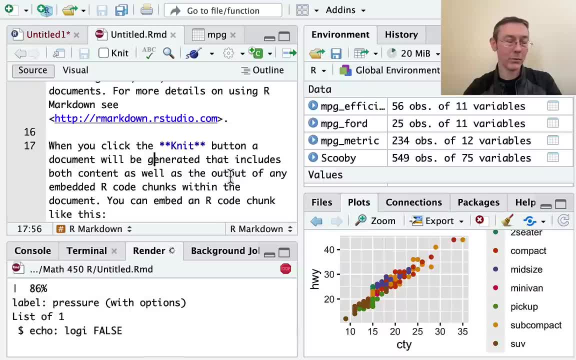 It's going to prompt me to save it, I will just take all of the defaults. Sorry, you didn't have to see my file structure there. It tends to move a little slowly. It's not the fastest thing in general, but in particular on my old computer. 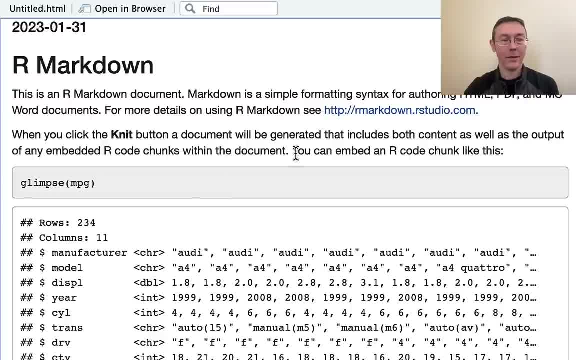 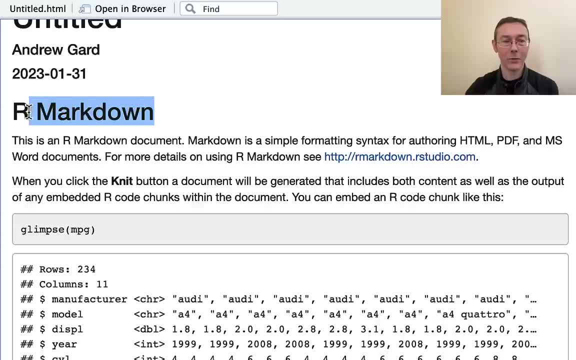 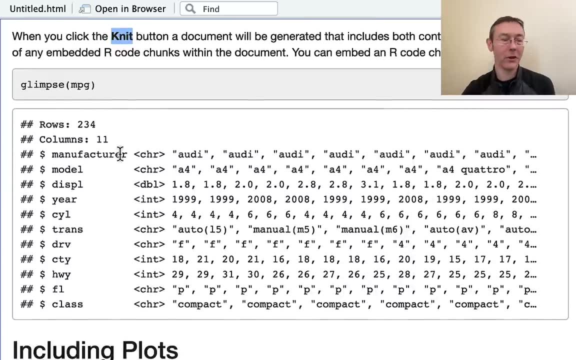 it is going to be really slow. There it is. You can see the name, the author and so on. I promised you a header here for our markdown, a link and some boldface. We got all of those: The code and the output of the code. 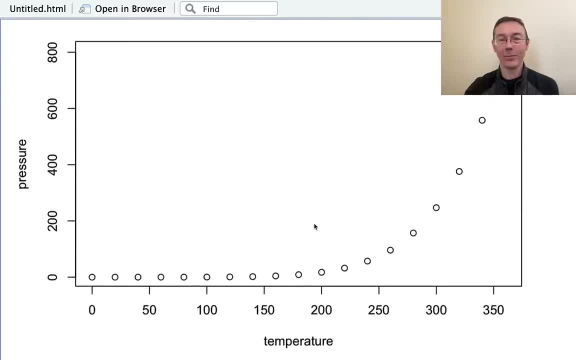 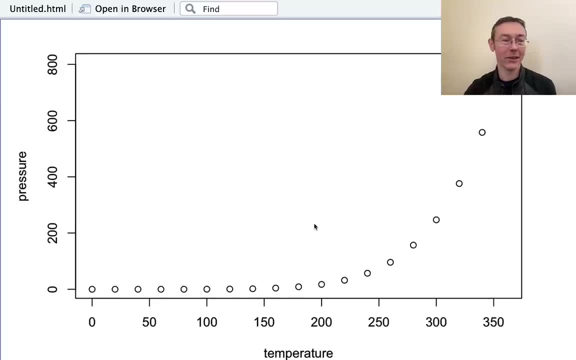 Right here And there's that old-fashioned plot. This does not look great in my mind. Possibly it looked great in the 80s when the function was written. These days it just looks kind of old-school. There are lots of different options. 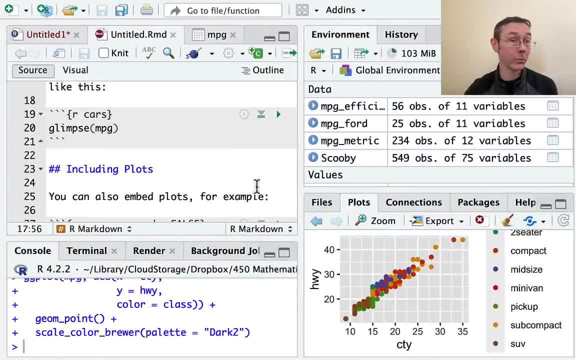 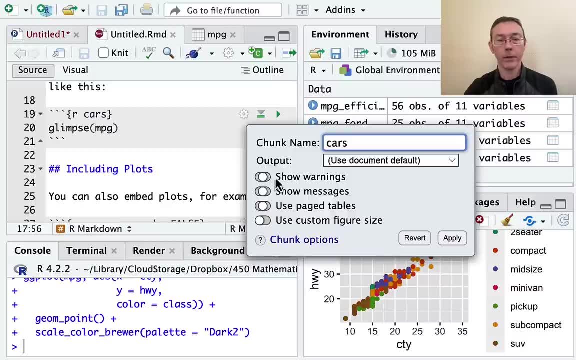 for these code chunks that you can explore as you get better at R. but I will just point out this little gear right here, And when you click on that gear you have choices. For instance, do I want to show the output of the code? 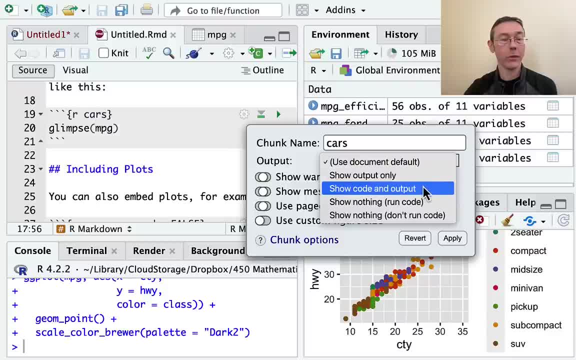 In this case the glimpse. so it was a table sort of thing. Do I want to show the code and the output, And so when you're writing reports for non-R users, for instance, you might want to suppress the code, But if you're writing,